An air parcel that's colder than the air around it is unstable, and that air parcel will rise on its own like a hot air balloon. An air parcel that's colder than the air around it is unstable and that air parcel will rise on its own like a hot air balloon. 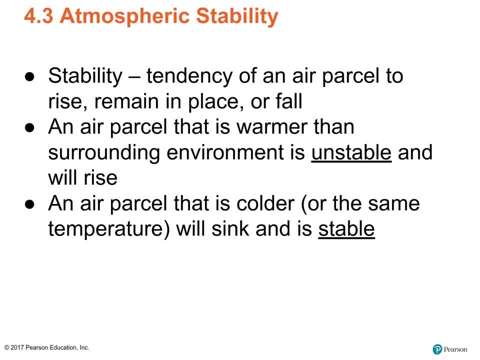 An air parcel that's colder than the air around it is unstable, and that air parcel will rise on its own like a hot air balloon. A hot air balloon and a parcel that's colder than the air around it will either stay where it's at or the air around it will either stay where it's at or the parcel will probably sink. so the air is stable. 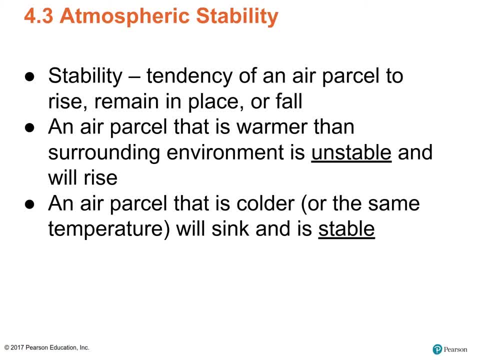 So really all we care about is: is it the parcel warmer than the air around it? If it's warmer, it will rise. If it's the same temperature or colder, it's not going to rise. we don't get rain as the atmosphere and the parcel are stable. 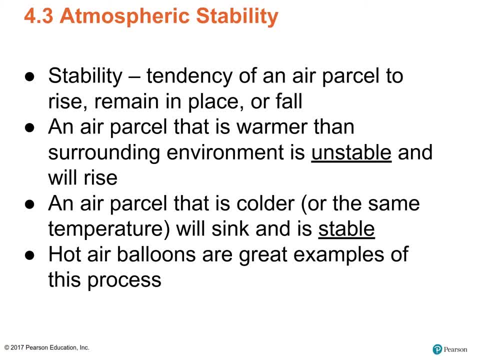 Hot air balloons are a great example. No one goes cold air ballooning because they don't rise. Hot air balloons rise because they're warmer than the air around it. warmer than the air around them and therefore the air is less dense, so it rises. 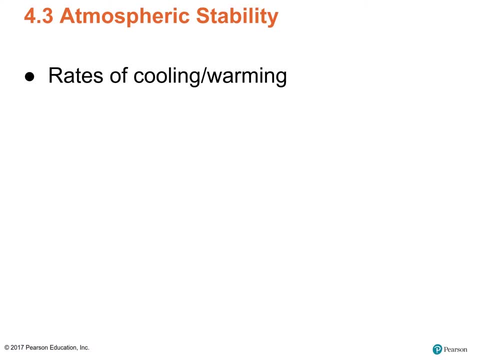 When we talk about rates of cooling and warming, we're going to be talking about two different categories. The first one is the unmoving atmosphere. There's two rates of cooling for this. Those are both lapse rates. So lapse rates refer to the change in temperature of the atmosphere. 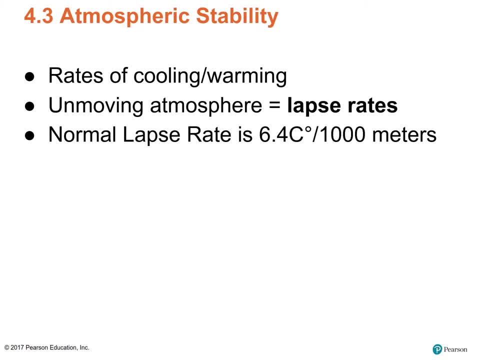 as you go up through it, There's the normal lapse rate, which we talked about before in the context of temperature profile in the troposphere. So as you go up through the troposphere, it gets colder by 6.4 Celsius degrees per kilometer, and that's the normal lapse rate. 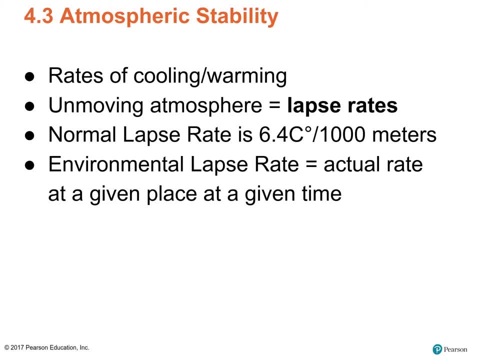 And then there's the environmental lapse rate, which is what it actually is. All over the world, hundreds of times a day, they send up weather balloons to try to calculate out the lapse rate and determine If the atmosphere is going to be stable, in which case it won't rain, or if it's going to be unstable. 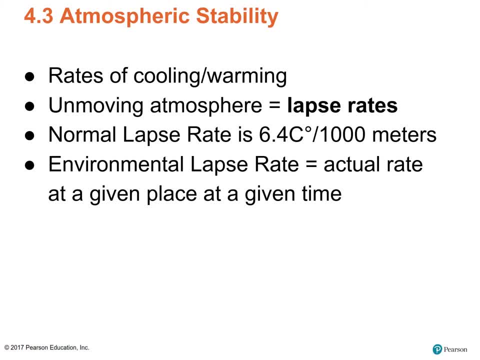 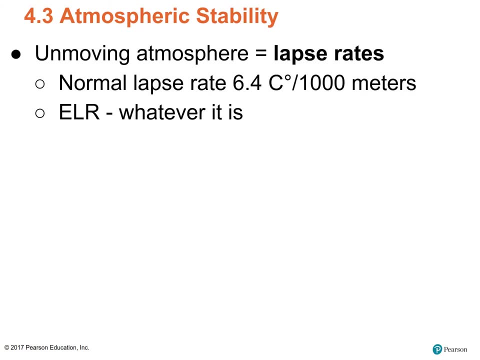 in which case you could get rain. If the atmosphere is really unstable, then you could get thunderstorms, lightning, hail, possibly tornadoes. So the more unstable the atmosphere is, the more extreme the weather is. So we have the lapse rates, the normal lapse rate, the environmental lapse rate and then 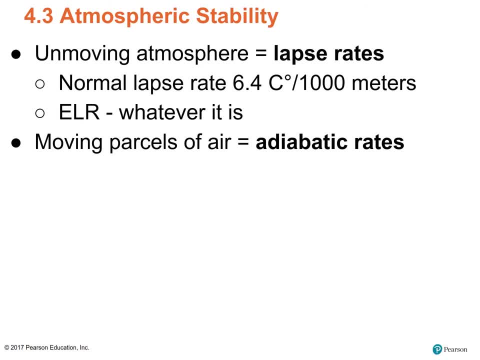 we have the rates that apply to moving parcels of air. Those are the adiabatic rates. There's the dry adiabatic rate, which is that a rising parcel of air will rise and cool by 10 degrees for every kilometer it goes up, and the moist adiabatic rate, which is 6 Celsius degrees of cooling for. 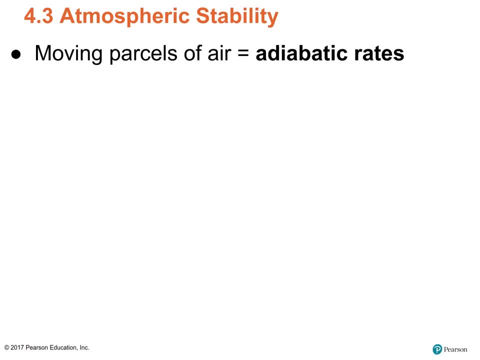 every kilometer the air rises. So more about the adiabatic rates. Adiabatic, the word itself, means a change in temperature without a loss or gain of heat. So in this case the air is cooling because it's expanding, not because of the temperature of the air around it. 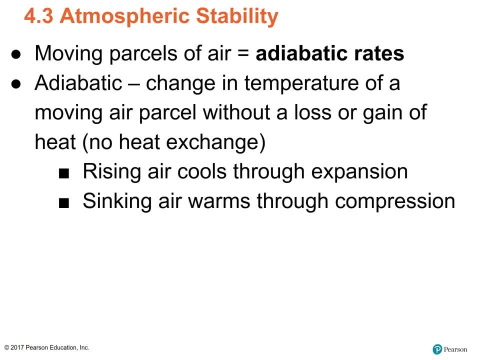 Rising air cools through expansion. Sinking air warms through compression. This is the idea behind diesel engines, for example. As you compress the fuel, air mixture gets hot enough until it ignites all on its own, and the heat is coming just from the air being compressed. So as air sinks, it gets. 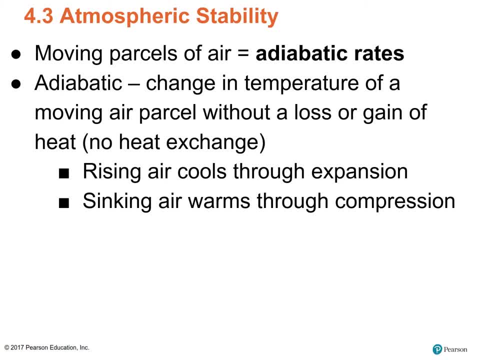 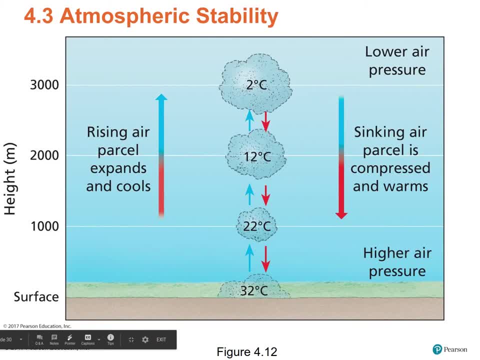 compressed and it heats up. As air rises, it expands and cools. So here we've got a diagram showing if we have air at 32 degrees at the surface and it gets lifted up, and it gets lifted at a kilometer, it'll cool 10 degrees to 22.. If we lift at another kilometer, it cools to 12.. 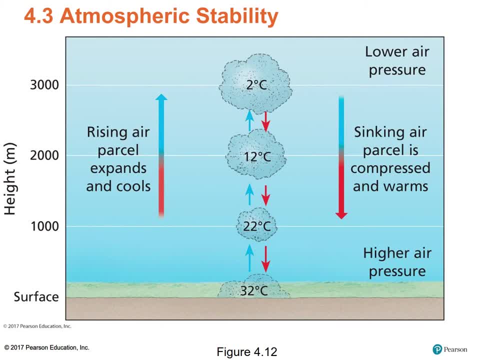 If we lift at another kilometer, it cools to 2. And the opposite is true of sinking air. So as the air sinks, it gets warmer by 10 degrees to 12,, warmer by 10 degrees to 22,, warmer by 10 degrees to 32.. 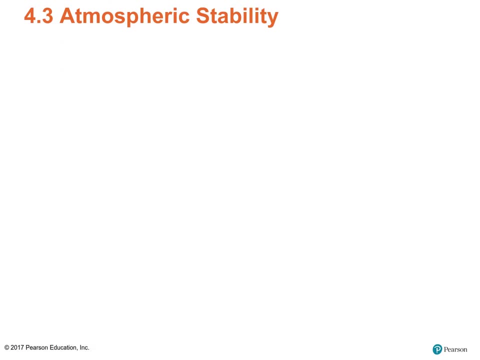 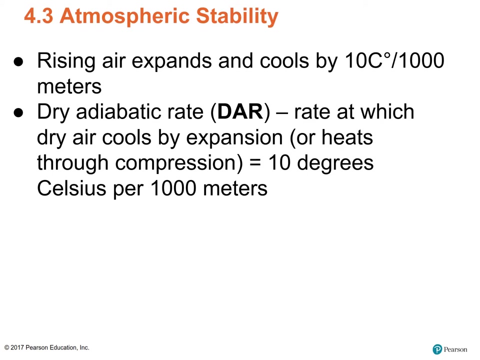 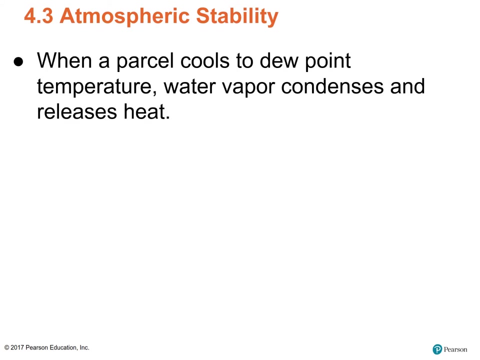 So rising air expands and cools by 10 Celsius degrees for every thousand meters it gets lifted. This is the dry adiabatic rate. That's the rate that dry air cools by expansion. Also, sinking air heats by compression: 10 degrees per thousand meters Once a parcel cools to dew point temperature. 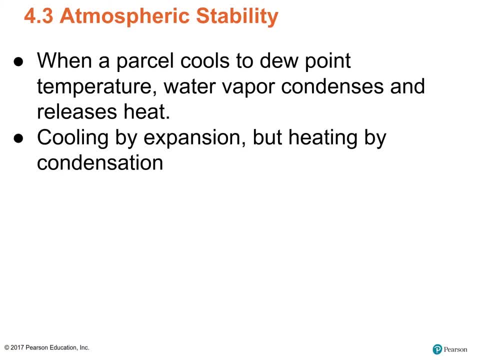 water vapor starts to condense and release heat. So within a parcel, as it rises and expands, it cools by expansion. but then as water vapor condenses, it releases heat. So the moist adiabatic rate is six degrees of cooling for every thousand meters of lifting. 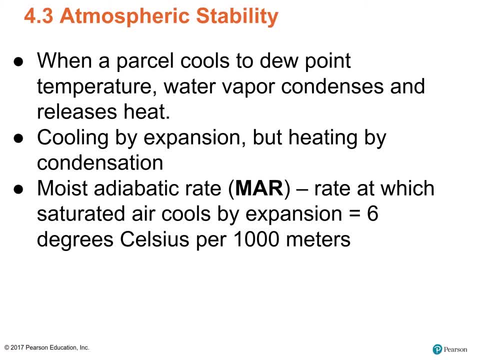 There's 10 degrees of cooling but then four degrees of heat released by the latent heat of condensation. The latent heat of condensation is one of the most important ideas in the whole chapter: The idea that as you put heat into water, it evaporates and then that energy is in the 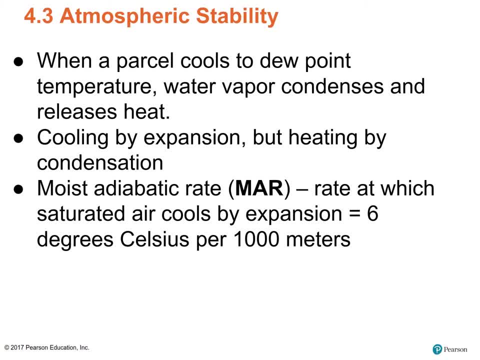 water. When the water condenses, the energy is released, warming the air around it. Once the air, as it's rising, cools to the dew point temperature and you get condensation, that altitude is called the lifting condensation level, although often we just abbreviate it as: 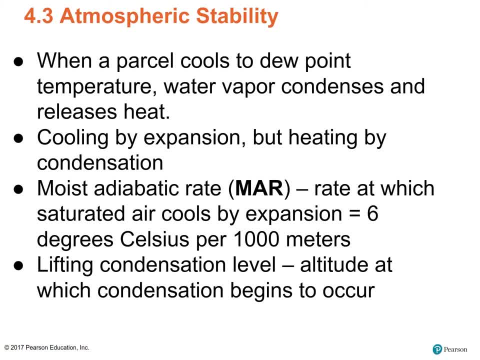 the LCL. So lifting condensation level is the height at which condensation begins to occur, And you can see this yourself as you walk around, If you look at clouds. this is why clouds have flat bottoms. As the air is rising, it's more or less uniform in. 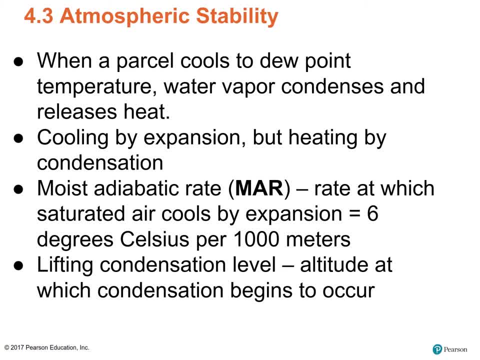 temperature and humidity, And so as it expands and cools, that's going to happen at about the same altitude as the air. So the air is rising, it's more or less uniform in temperature and humidity, And so as it expands and cools, that's going to happen at about the same altitude. 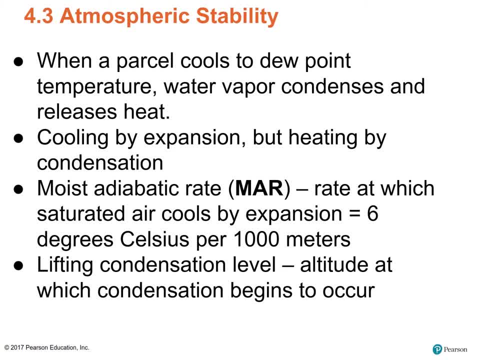 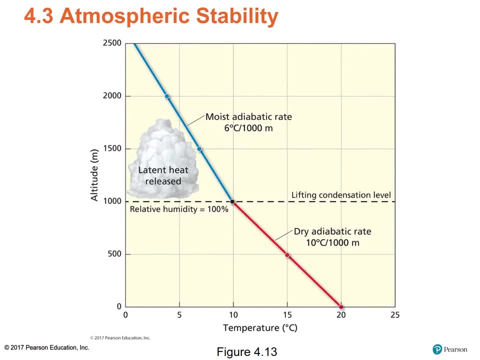 so you get flat bottoms on clouds Once the air hits condensation, once it cools to dew point temperature. as it keeps rising, it's still going to remain at dew point temperature. So clouds are bumpy on top but they're flat on the bottom. Here we have a diagram showing how air is going to cool. 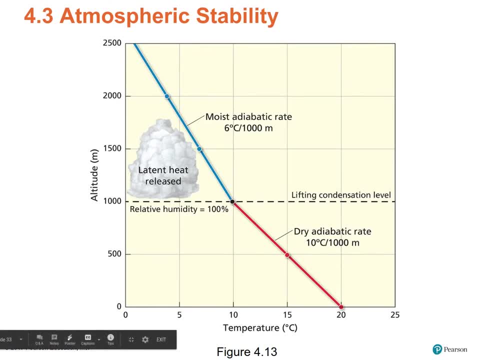 as it rises, starting with 20 degrees at the surface. If we have a parcel of air that we lift up a kilometer, it's going to cool by 10 degrees and in this example our dew point temperature is 10 degrees. It hits 100% relative humidity. you get condensation which releases heat. So now once 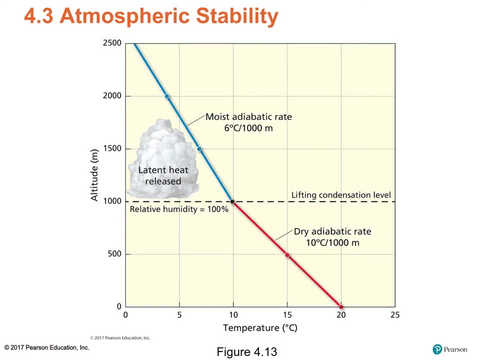 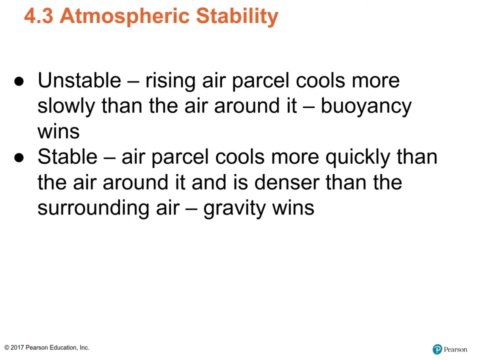 you've hit 100% relative humidity at the dew point temperature. the parcel is going to cool at the moist adiabatic rate of 6 degrees. If the rising air parcel is warmer than the air around it, it's unstable If the air parcel is cooler or the same. 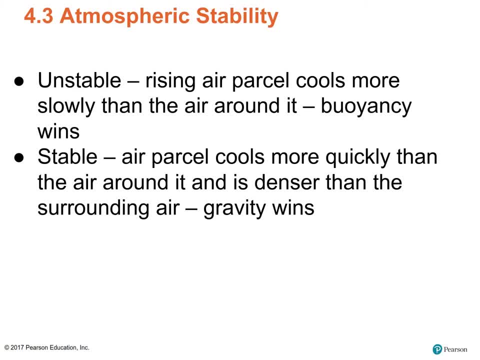 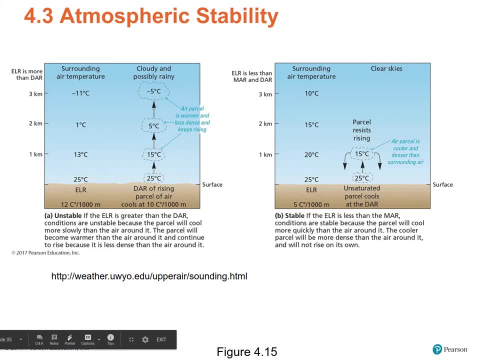 temperature, then it's stable and it won't rise on its own. So here we have two examples: looking at a parcel of air, cooling at the dry rate and in this case we have an environmental lapse rate of 12.. So the air, the atmosphere, as you go up- every kilometer you go up, it gets colder by 12 degrees, down to 13,. 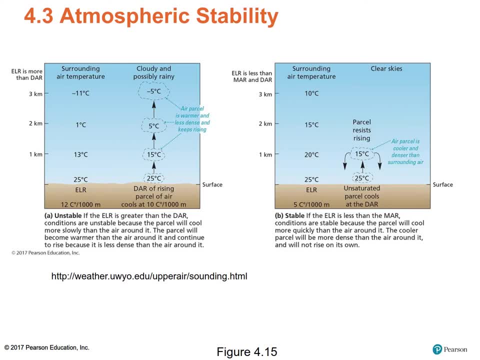 12 degrees down to 1. 12 degrees negative 11.. Our parcel is cooling at 10 degrees. so every kilometer you go up, the parcel cools by 10, but the air around it cooled by 12.. So they were the same temperature but at 1 kilometer. 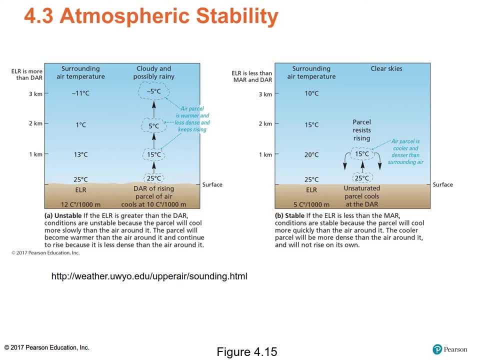 the parcel is 2 degrees warmer. If we lift at another kilometer we'd see the atmosphere that's not moving. cooling at the ELR has cooled to 1, our parcel is cooled to 5, so now it's 4 degrees warmer. If we lift at another kilometer, it's going to get another 2 degrees warmer. so now it's 6 degrees warmer. 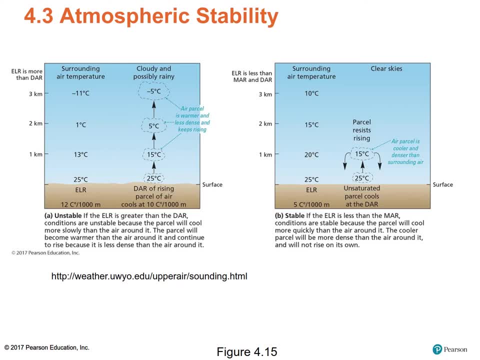 than the air around it. You can see in this example, as we keep lifting it, it will become warmer relative to the air around it. It'll get warmer relative to the air around it. It's cooling the whole time, but it's cooling more slowly than the air around it, So it's 2 degrees warmer. 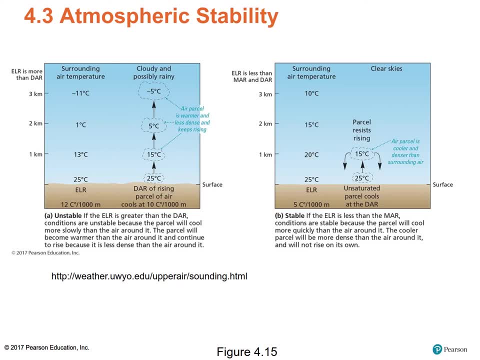 it's 4 degrees warmer. it's 6 degrees warmer As our parcel rises. it's getting more and more unstable as it gets relatively warmer than the air around it. On the other hand, if the ELR is low, for example 5 degrees, we start off again with the same temperature: 25, 25.. If we lift that, 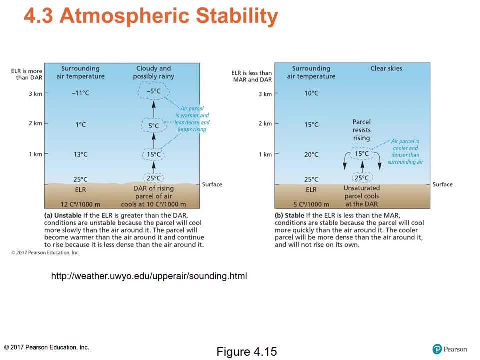 parcel a kilometer. our parcel cools by 10 degrees down to 15, but the air around it, since the ELR is 5 degrees of cooling, is going to cool to 20 degrees. So now our parcel is 5 degrees colder than the air. 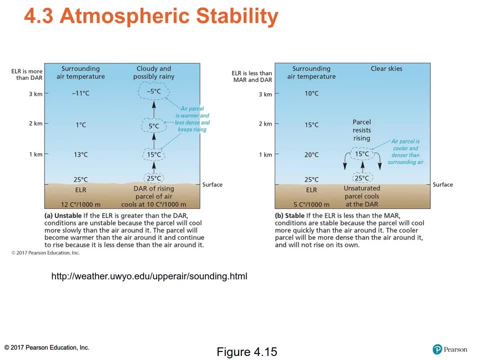 so it's going to resist rising. it's not going to rise unless it gets lifted up by a mountain. Without a mountain, though, the atmosphere is going to be stable, the parcel is not going to rise. we're not going to get rain. 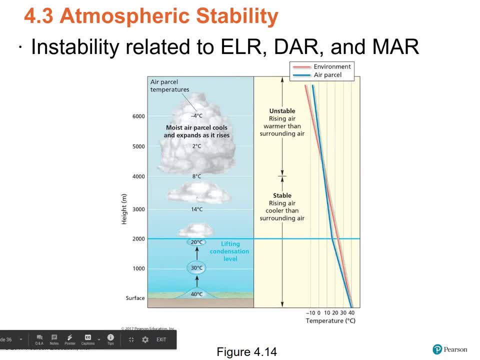 In this diagram we have a parcel of air that's rising and cooling at the dry rate up to the dew point temperature. You can see the ELR here is 8, the dry rate is 10, so the atmosphere is cooling off a. 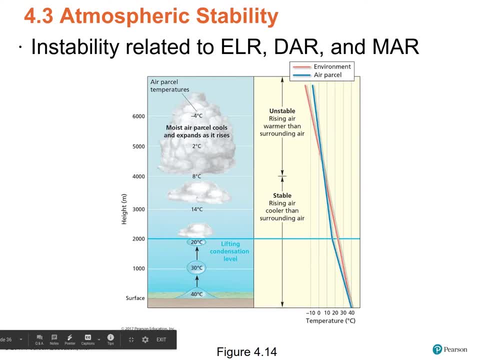 steady 8 degrees per kilometer. Our parcel starts cooling off at 10 degrees, so by the time it's up to 2 kilometers, it's going to be 4 degrees colder than the air around it, so it would be stable. 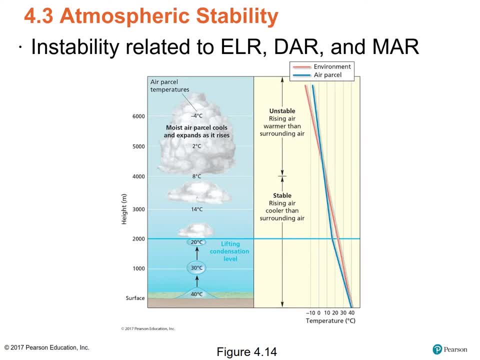 If, however, that air parcel now hits the condensation, the lifting condensation level, it's cooled to dew point temperature now it's going to cool by 6 degrees. the air around it's going to cool by 8.. So if that parcel, for example, gets lifted by a mountain, if it rises another 2 kilometers, 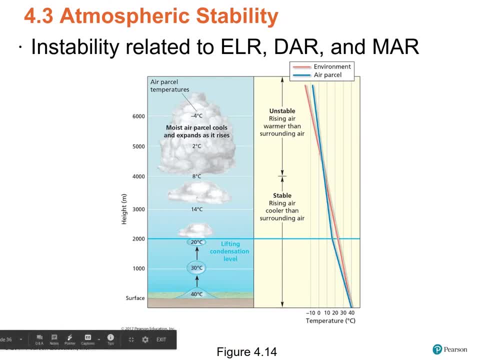 now they'll both be the same temperature, because our parcel started cooling by 10 for 2 kilometers and then by 6 for 2 kilometers. The atmosphere, though, has been cooling at 8 the whole time, Above 4 kilometers. our parcel is going to be warmer because it's cooling by 6 degrees. 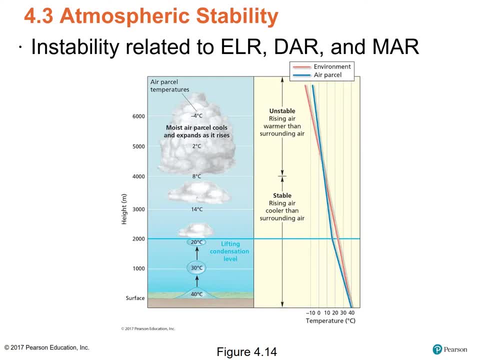 the atmosphere is cooling by 8 degrees, so above 4 kilometers our parcel is going to be unstable And you can tell by looking at the chart. the temperature of the parcel is on the right-hand side. the right-hand side is the warmer side of the temperature profile. 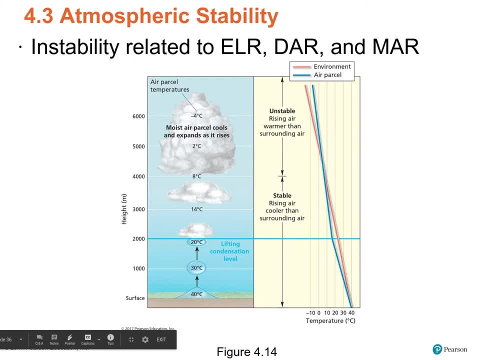 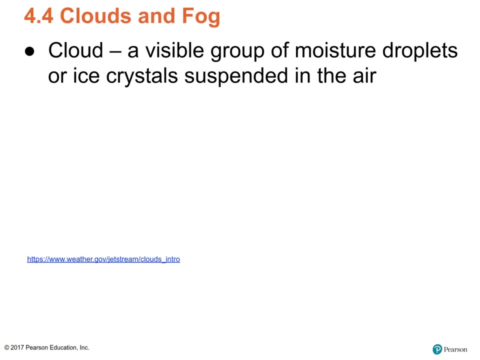 So above 4 kilometers you can see the blue line is to the right of the red line. so the atmosphere is colder than our parcel. So if the parcel is warmer than the air around it, it's unstable, Clouds and fog. 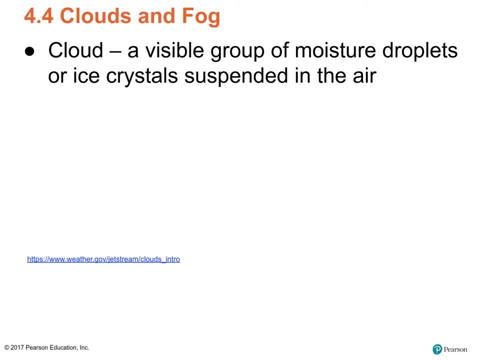 A cloud is just moisture droplets or ice crystals suspended in the air. If it's on the ground, we call it fog, And I've included down here a link to the National Weather Service's Jetstream site, which is one of their educational sites. you can go there and read about clouds, how they're. 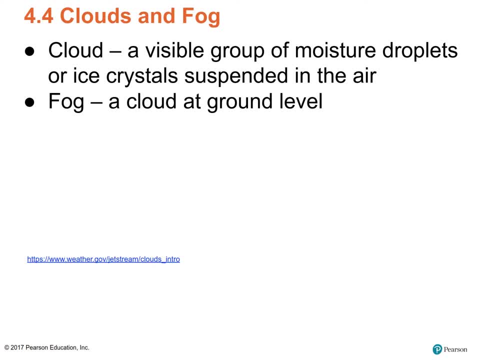 formed what the different clouds can tell you about the environment. I hope you check it out. you could learn some stuff and it's fun. Precipitation is just liquid or solid water, so that's rain, snow, hail falling from the 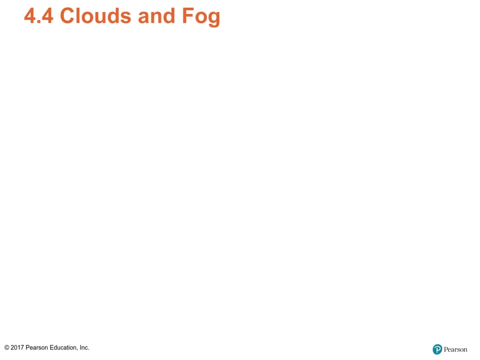 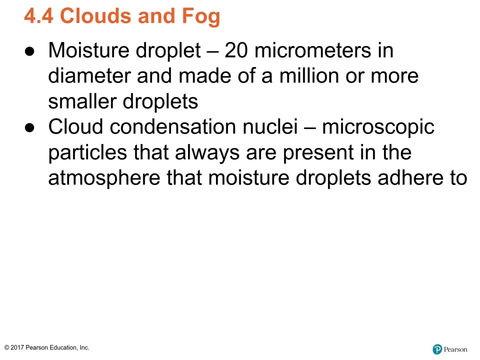 clouds. Often we just call that precip for short. Clouds are made of moisture droplets. Those are made of droplets which are even smaller droplets. Those droplets form on cloud condensations. They're made of water. Cloud condensation nuclei. 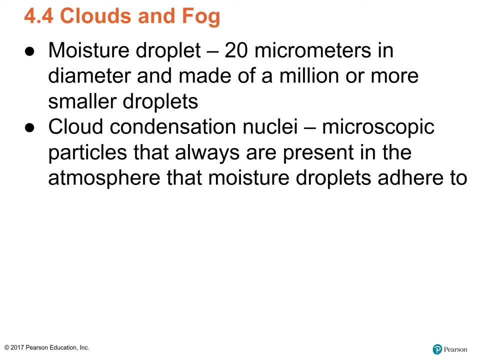 In order for water vapor to condense- and this is really weird, I yeah, it's just weird- Water vapor needs to condense out onto something. So water vapor when it condenses, you might have seen water vapor condensing out onto. 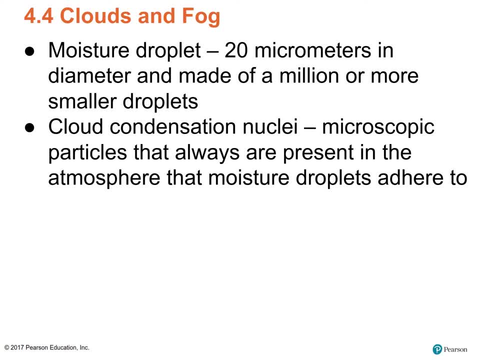 a glass. if you have a drink with ice cubes in it, It's condensing out onto the glass, not the air by the glass. That would be really cool. You could have a little cloud around your glass, but that doesn't usually happen. 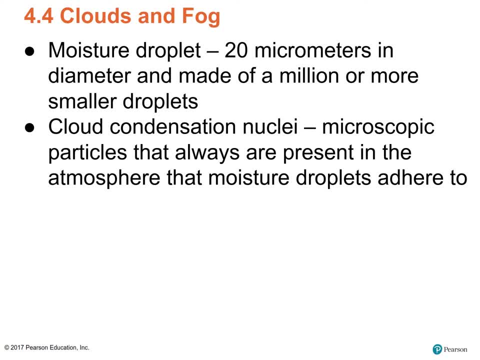 So water vapor condenses out on these things called cloud condensation nuclei. Cloud condensation nuclei: Those are microscopic particles. There's probably a billion in every cubic meter of air that we are used to. They're made of soot, dust, ash, pollen, smoke. 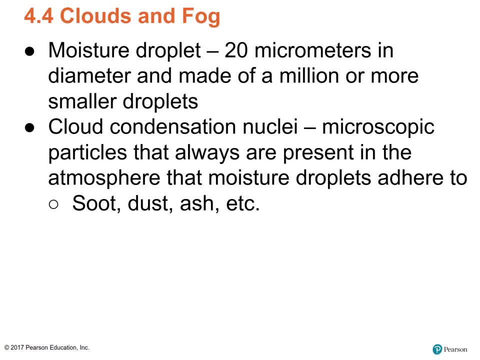 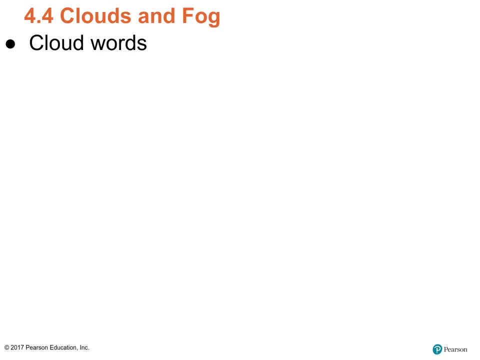 All of those act as cloud condensation nuclei. So to for water vapor to condense, you need to have saturated air and cloud condensation nuclei. These are some cloud words. Luke Howard is the scientist back in the 1800s. 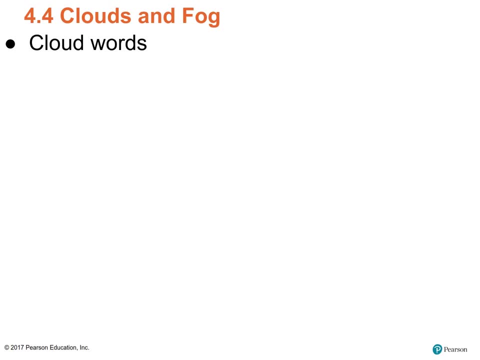 That cloud condensates. He classified clouds. He was an amateur naturalist and he thought it would be a good idea for science to classify clouds in the same way that they were beginning to classify living organisms. And his clouds have Latin root words. 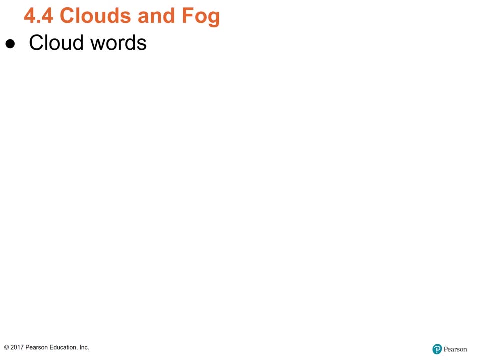 So if you didn't grow up speaking Latin, these words are probably new, And I think if you learn the words, it'll help you understand the clouds and remember them better. They're not just nonsense words. So the first one, cirrus. 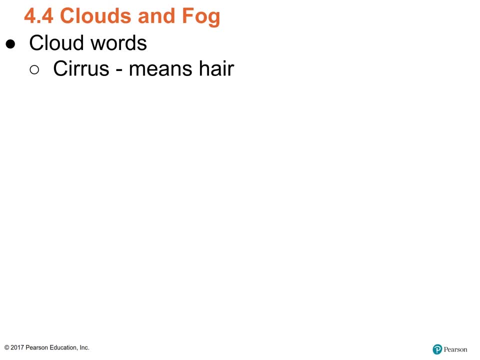 Cirrus means hair like wispy Cirrus clouds are made of ice crystals and they have this distinctive wispy appearance. Cumulus means heap or pile, little puffy cotton ball clouds or cumulus clouds. Stratus means layer. Alto is the prefix for two of the mid-level clouds: alto-stratus, alto-cumulus. 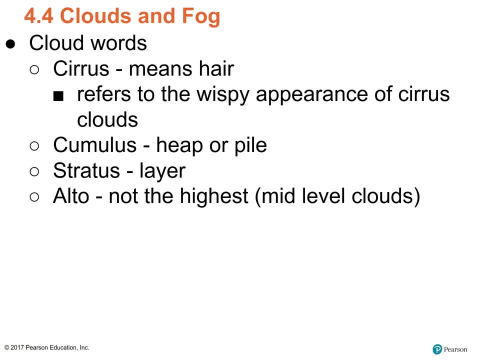 Alto means not the highest, So the highest are cirrus, cirrostratus, cirrocumulus, and then the mid-level clouds are alto-something, alto-cumulus, Alto-cumulus, alto-stratus. The word nimbus means rain, so cumulonimbus means pile of rain. 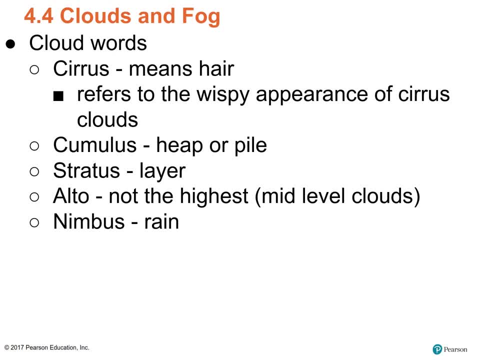 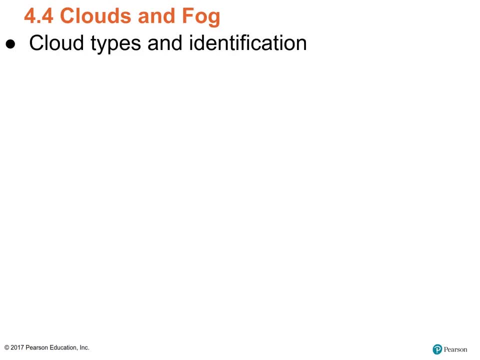 The thunderclouds are piles of rain. Nimbostratus would mean layer of rain. Harry Potter's broom was a nimbus 2000.. So Luke Howard divided clouds into three categories, actually four. He had high clouds. Those are above 6,000 meters. 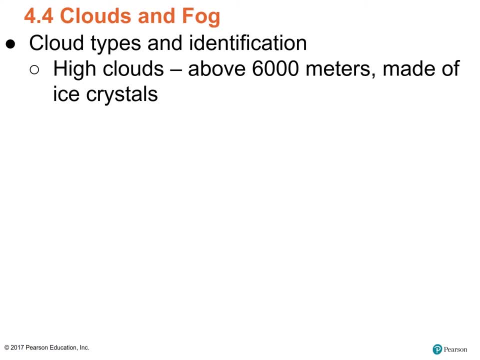 They're made of ice crystals. They have a distinctive appearance. We'll talk about that in a minute. There's the mid-level clouds, The alto clouds, And then there's the low clouds. Those go from the surface up to about two kilometers. 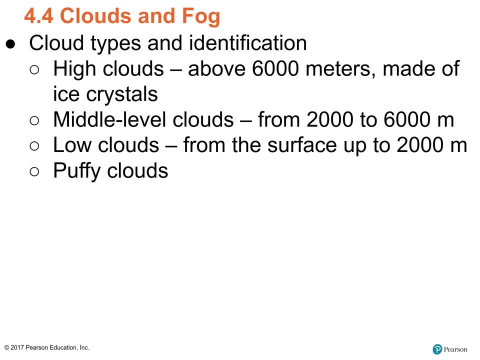 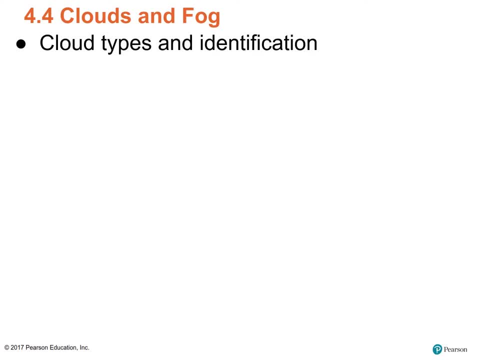 And then puffy clouds, although really it's just the cumulonimbus cloud, and those go from the surface up to six to 10 kilometers, So they really transcend the divisions of altitude. So we have the high clouds, Those are above 6,000 meters. 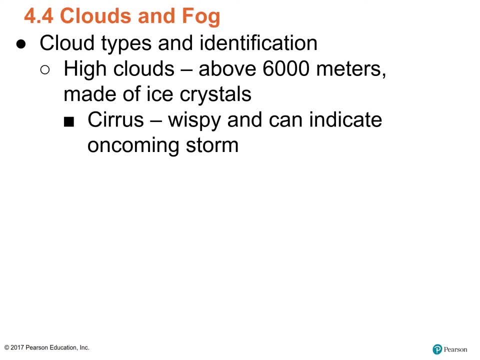 They're made of ice crystals. The most important ones probably are cirrus. Those are wispy Cirrus clouds tell us that a storm is probably coming in 24 hours. So if you see these wispy cirrus clouds, it's an indication that a storm is coming. 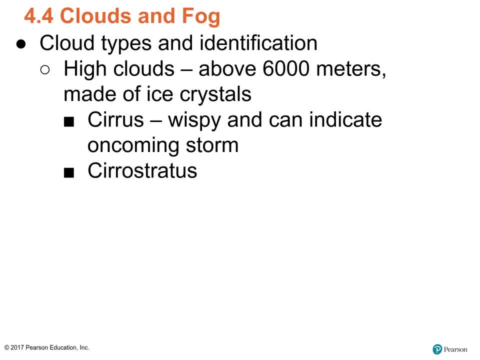 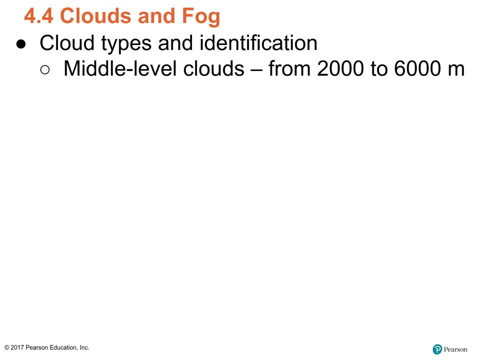 Or rather it can be. Cirrostratus is a layer of hair And then cirrocumulus means little piles of hair. The mid-level clouds are alto clouds, So altocumulus means mid-level, little piles. Altostratus is a flat layer. 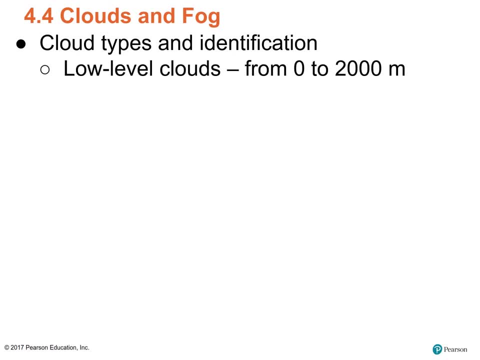 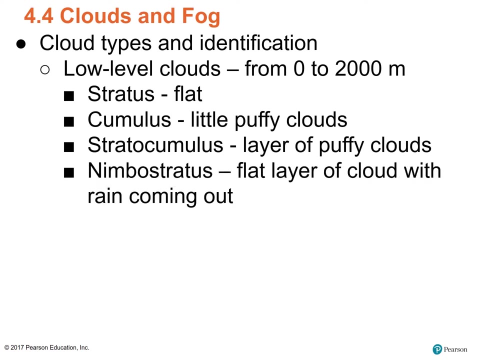 It's very boring. For the low clouds we have stratus Flat, probably the most boring of all- the clouds Cumulus, little puffy clouds, Stratocumulus, which is a layer of little puffy clouds, Nimbostratus. if it's flat with rain coming out, it's nimbostratus. 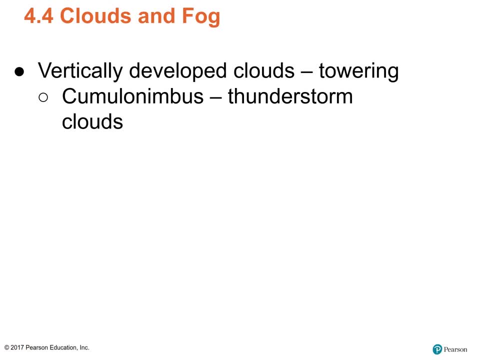 And then the vertically developed clouds, The towering cumulonimbus, the thunderstorm clouds. we'll talk about them in a minute. They produce lightning, They produce thunder, wind gusts, They have ice crystals and frozen water in them. They can, if they get large enough, they can, develop tornadoes. 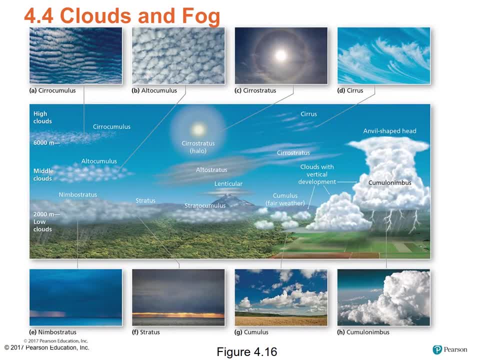 And here's a good diagram of cloud types. So, starting with the highest clouds, we have cirrus clouds, the wispy, wispy, wispy cirrus clouds, Cirrostratus, shown here with a halo. Ice crystals refract or bend the light from the sun. 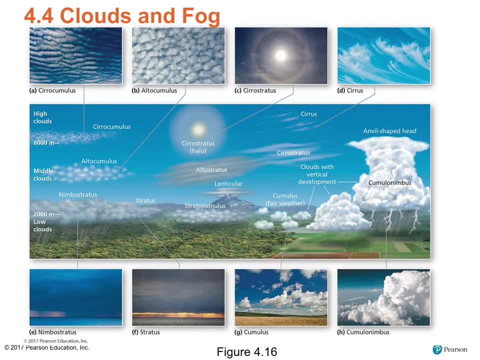 So cirrostratus, cirrus and cirrocumulus clouds. you can get this distinctive halo and that tells you that the clouds are made of ice crystals. So we have cirrus, cirrostratus, cirrocumulus. 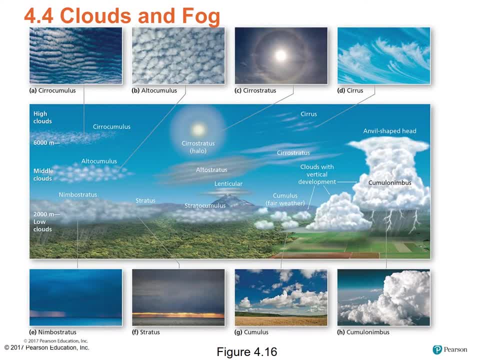 For the altoclouds, we have altocumulus, little puffy clouds, a layer of little puffy clouds. Altostratus, let's use just a flat layer. Nimbostratus, it's a layer with rain coming out. 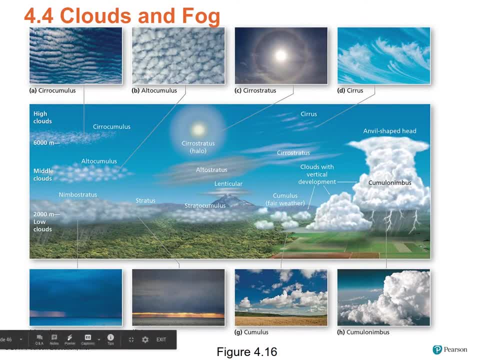 Stratus, it's just flat. Cumulus- the little puffy clouds- I think we've all seen those- And then cumulonimbus are the largest. They can go from just a couple hundred meters off the ground up to, like I said, 10,000. 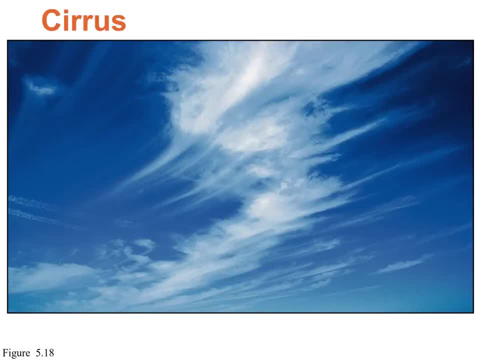 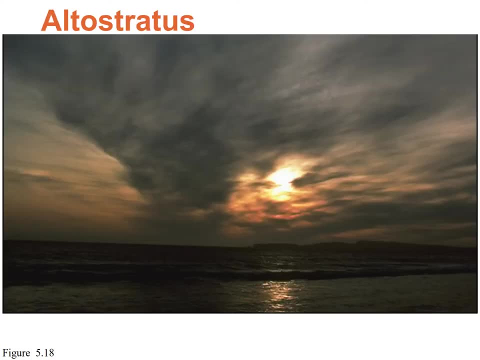 feet in the air. Let's look at some close-ups though. We have cirrus, the distinctive wispy ones. Altostratus- it's a boring flat mid-level layer Altocumulus- they're puffy. 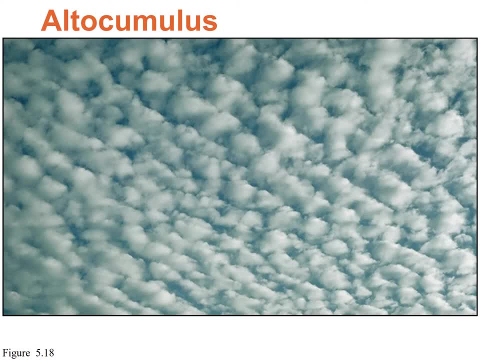 They're not made of ice crystals and we can tell because they look like little cumulus clouds. So they're farther up in the sky, they're higher in the sky, but they're not made of ice crystals, They're altocumulus. 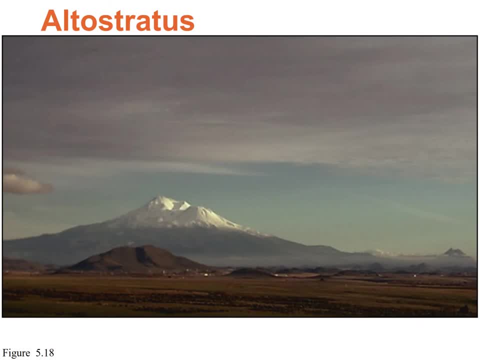 Altostratus- again the boring flat layer. In this case it's over Mount Shasta. We'll see Mount Shasta. a lot People really like taking pictures of Mount Shasta with clouds on top of her Stratus. it's just a layer. 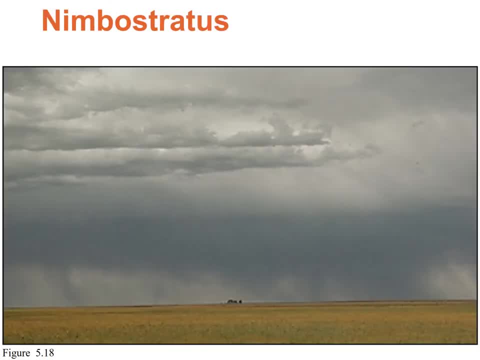 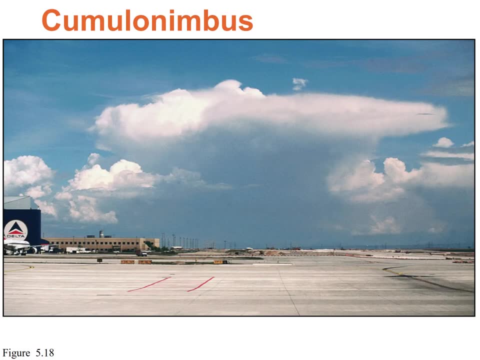 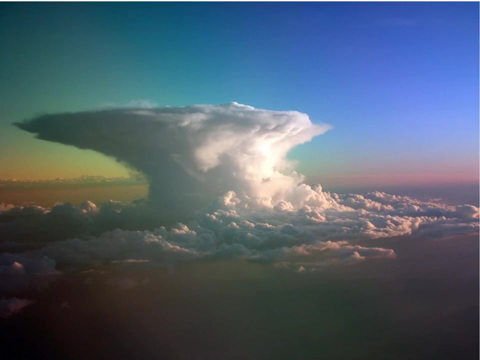 It's boring Nimbostratus, at least there's rain coming out of it. Cumulus- little puffy cotton ball clouds, And then cumulonimbus. These are the largest clouds. Here is a cumulonimbus cloud taken in flight from an airplane. 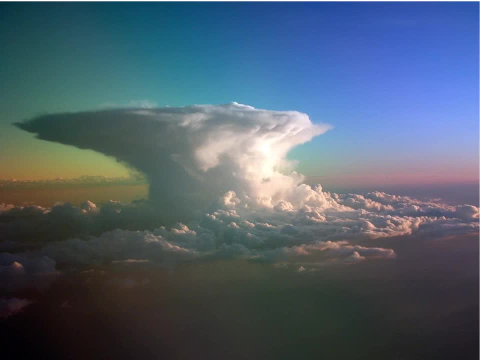 You can see cumulonimbus clouds have this shape. They're not made of ice crystals. They have this distinctive flat top. They're often called anvil clouds, you know, like the anvils that Wile E Coyote drops on his head. 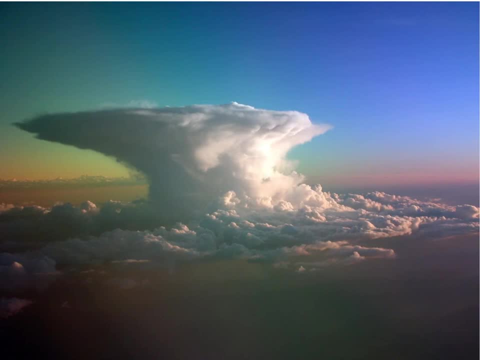 And what happens is as the air is rising. it's rising because it's warmer than the air around it, until it runs into the top of the troposphere, the tropopause. and at the top of the tropopause there's the isothermal layer, where the ELR goes to zero. 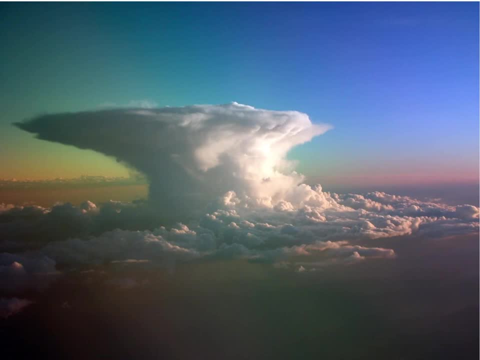 So the air temperature here is the same as the air temperature here. As the air rises in the cloud, though, the air in the cloud, as it rises, expands, and then it goes up, It expands and cools. So as it rises and cools, it's colder than the air up here, so it can't rise anymore. It's like an inversion layer almost, And the other reason that the cumulonimbus clouds get flattened off is by the jet stream. So high winds in the jet stream make them flat and they also flatten as they run into the isothermal layer at the tropopause. 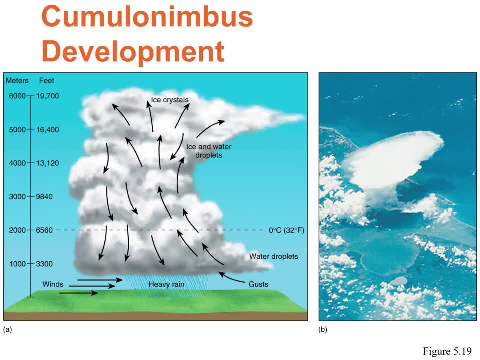 To make a cumulonimbus cloud. there's a positive feedback loop. that has to happen. As the air rises, it expands and cools. You get condensation, which releases heat, which warms the air a little bit, so it keeps. 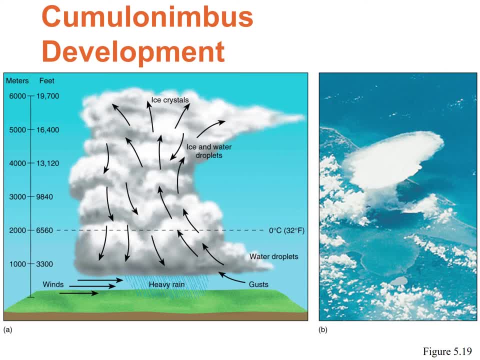 rising And that happens again. As it rises it expands and cools, which causes condensation, which releases a bit of heat. so it keeps rising. As it does that it's going to pull in more warm, moist air. 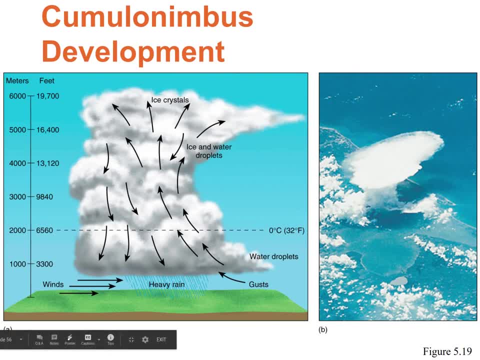 And that process is, like I said, like a feedback loop: The bigger it gets, the bigger it's going to get. Here's another cumulonimbus, This one's over Florida, taken, I think, from the space station. 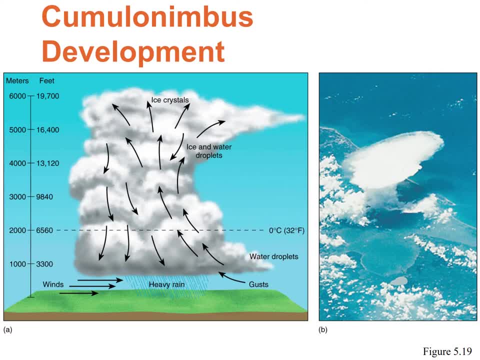 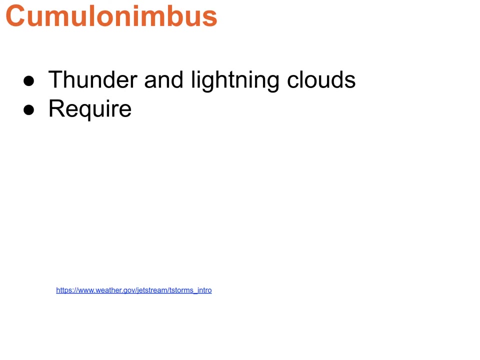 And you can see the distinctive flattening out, almost like the air has hit an invisible barrier, which it has, And that invisible barrier is probably the isothermal layer at the top of the tropopause. So cumulonimbus are thunder and lightning clouds. 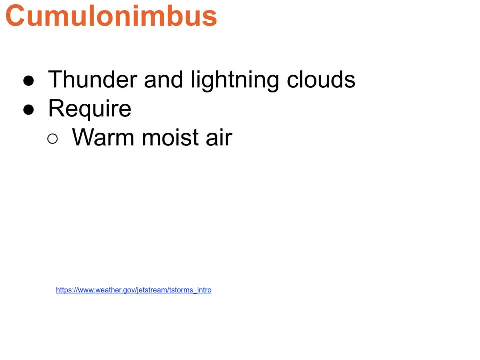 To make them you need lots of warm, moist air. Remember it's that latent heat of condensation that powers cumulonimbus clouds. As the water vapor condenses, it releases heat which warms it. You need a very high ELR so, as your air is rising, it's cooling more slowly than the 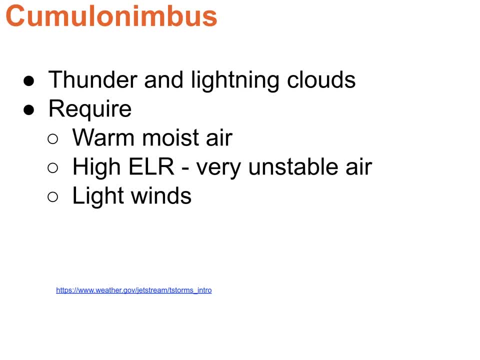 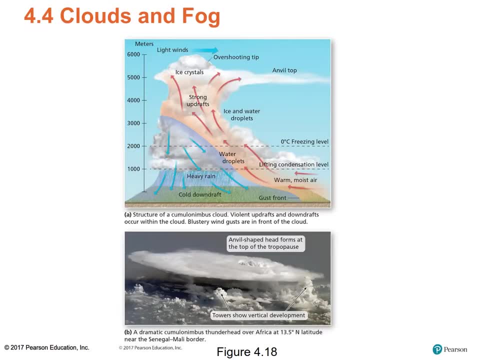 air around it And you need light winds to keep the storm moving along, otherwise it would run out of warm, moist air. Here is a diagram- another diagram- of a cumulonimbus cloud showing the lifting condensation level, Again flat-bottomed. 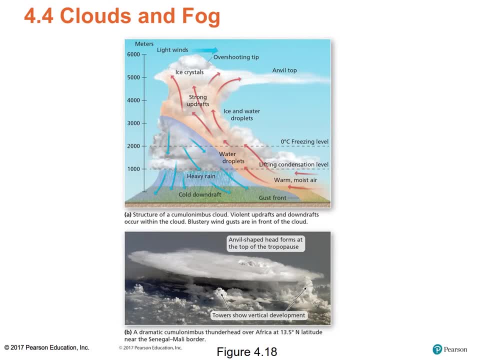 Here's the freezing level. So as the air rises, it's going to expand and cool. You'll get condensation. So down here the cloud's made of water droplets, Here it's made of ice droplets, And this is how we get hail. 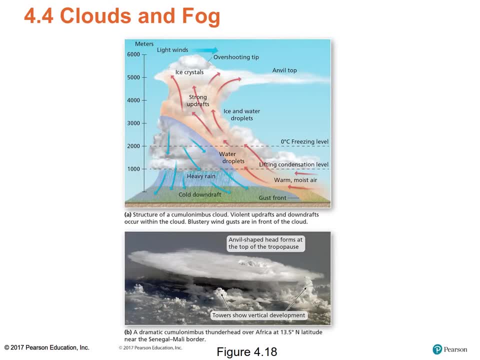 The air as it rises and the water, the rain, instead of falling down, because there's these updrafts, and the updrafts can hit 125 miles an hour straight up. So as the water gets picked up, it freezes, becomes hail, and as it falls down, it'll. 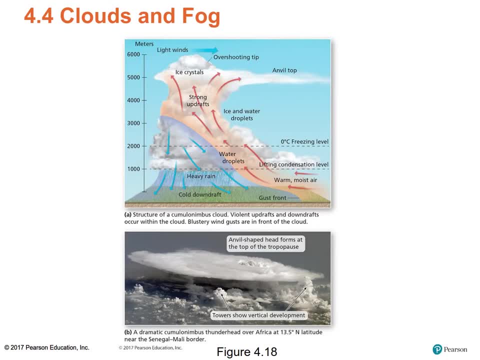 often get picked up by another updraft, and it can make several trips around, And so the hailstones get bigger and bigger and bigger. This one is. this picture here is an example of a cumulonimbus cloud over the Senegal-Mali. 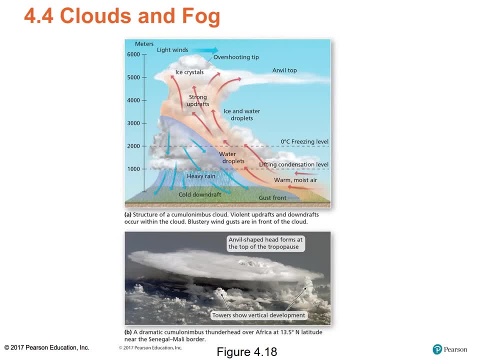 border. This was again taken from the space station, So you can see little little convection towers, little little hot towers of air as they're rising in the cloud, and then the cloud spreading out when it hits the isothermal layer. 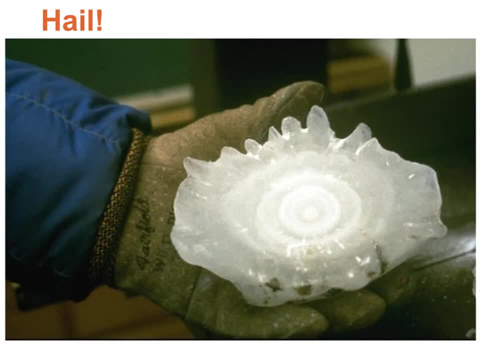 This was, at the time, the largest hailstone ever recorded. It weighed 1.75 pounds. It was the largest hailstone ever recorded. It weighed 1.75 pounds. It was 18 inches in diameter. It fell in Coffeyville, Kansas. 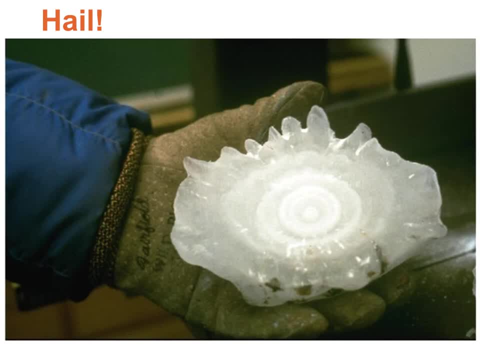 And you can see. it's got many layers. It's been cut in half so we can see them And it looks like it's made. there's one, two, three, four, at least five, well six, seven trips up and down through a thunderstorm. 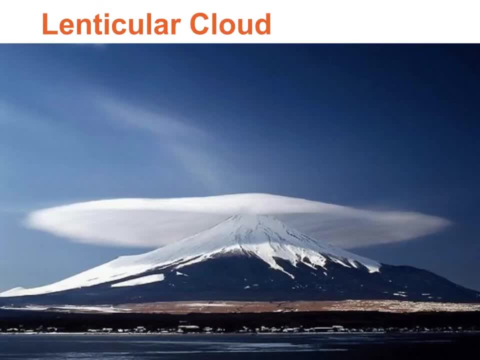 It's finally fell to the ground. This is a lenticular cloud over Mount Fuji. Lenticular clouds are Except for the fact that they're both clouds. They're both clouds, the exact opposite of a cumulonimbus cloud. 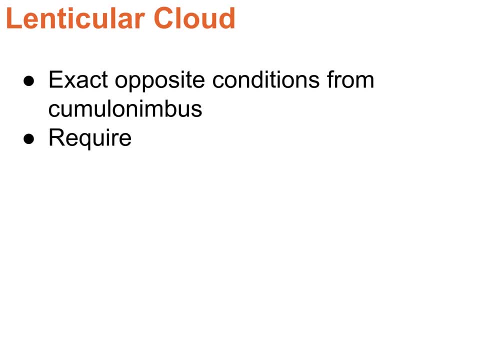 So to make a lenticular cloud you need to have warm, moist air, a physical barrier to lift air up, in this case a mountain. You need to have a very low ELR, so the air has to be stable. 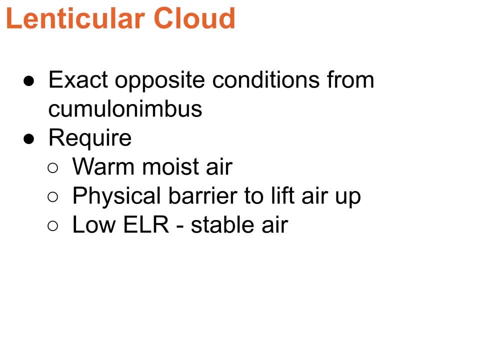 As the air is rising, it expands, it cools, you get condensation which releases heat, but the air around it is still warmer, So the parcel is stable. It's not going to keep rising as soon as it runs out of mountain. 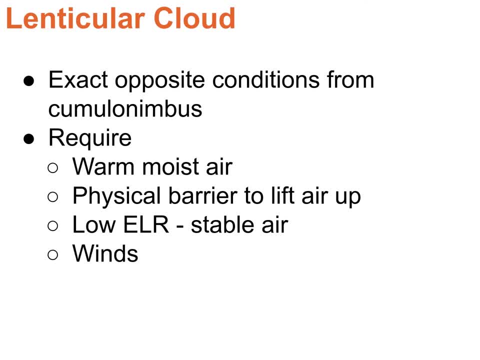 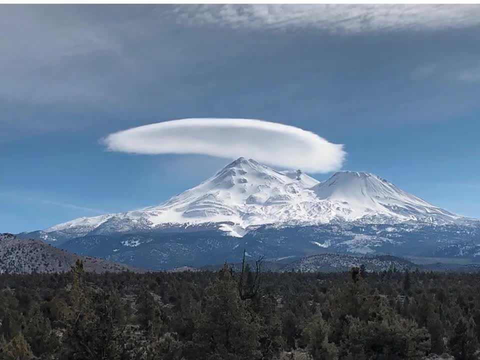 The air is going to sink. heat up, the cloud's going to evaporate. You also need winds. The winds are what is pushing the air up the mountain, to make it expand and cool. So here again, I promised more Mount Shasta. 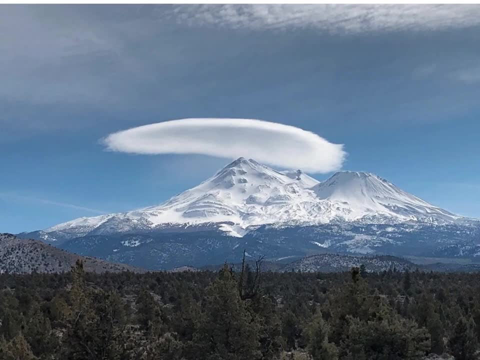 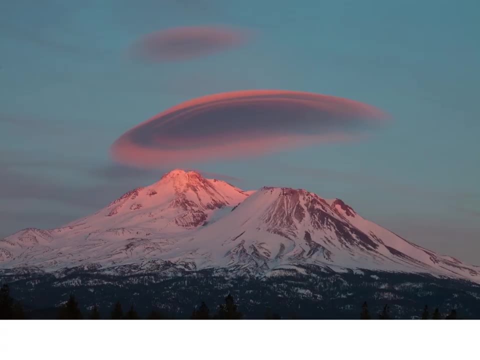 Here you can see a lenticular cloud over Mount Shasta. The air is rising, expanding, cooling, and then, as soon as it runs out of mountain, it sinks and evaporates. Another shot of Mount Shasta showing a deep cloud. 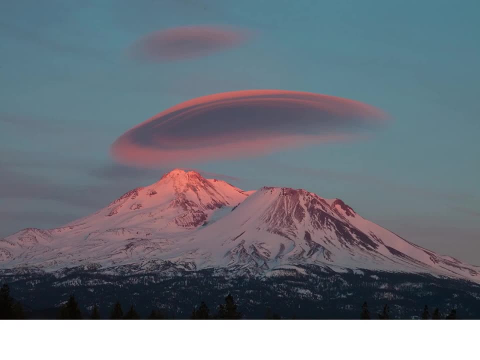 Coming a different day with a different lenticular cloud And, as the day goes on, this will just hover over the mountain, although the droplets of water that come in condense and then evaporate. So really you're not seeing a cloud, you're seeing a region of condensation that stays. 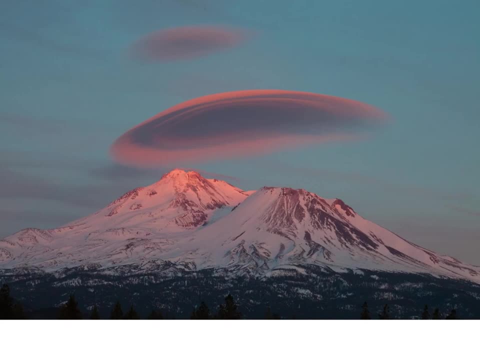 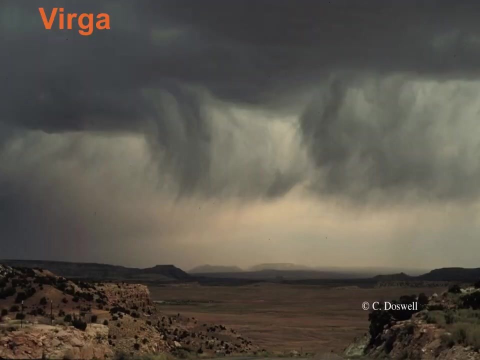 in place. The actual physical particles are coming and going, but the cloud stays in place, although it's not the same cloud, because the water droplets keep moving. Virga- This is just a vocabulary word Word for rain that falls from a cloud that evaporates before it hits the ground. 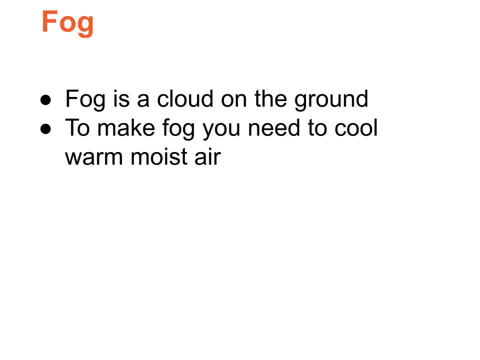 Fog is a cloud on the ground. In order to make fog, you need to cool warm moist air. So there's five kinds of fog and they're all classified based on what does the cooling? We've got warm moist air. something's going to cool it. 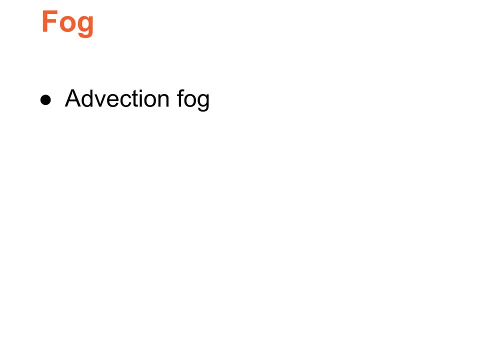 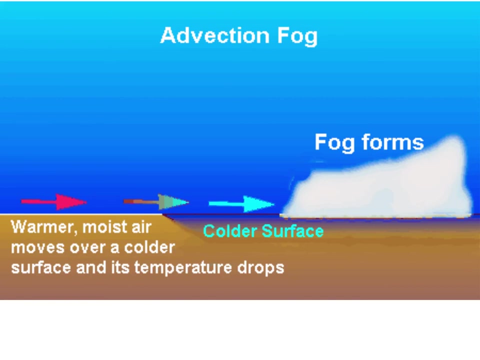 That's what determines the five types of fog. So we have advection fog, Evaporation fog, Upslope fog, Valley fog And radiation fog. Advection fog is caused by advection. Advection is just a fancy word for wind. 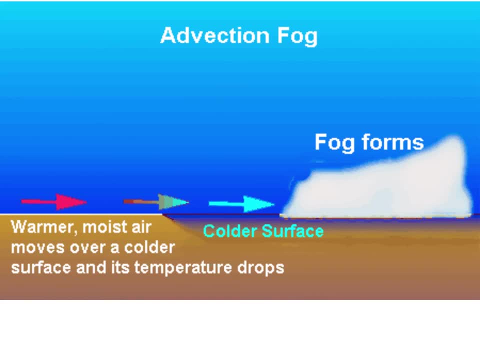 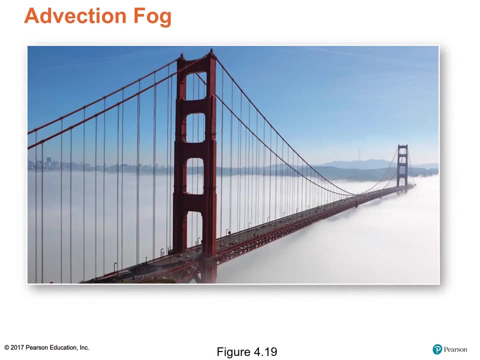 Air blows sideways. Our parcel of air goes over a cold surface. it gets cold and you get fog. So San Francisco's fog is caused by warm air getting blown over the cold ocean. The air gets cool, you get condensation. bada boom, bada bing. you got advection fog. 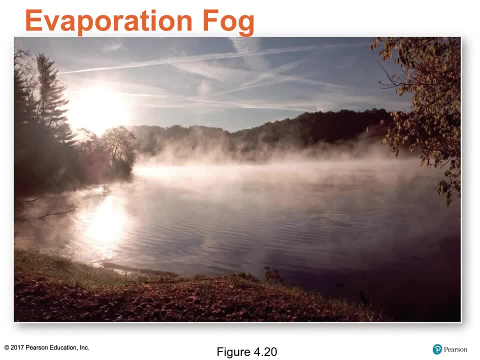 Evaporation Fog. Evaporation fog happens when you have water that is slightly warmer than the air above. So this is Donner Lake, so the water is pretty cold, but the air above it is even colder. So the water evaporates, hits the cold air, condenses and you get fog. 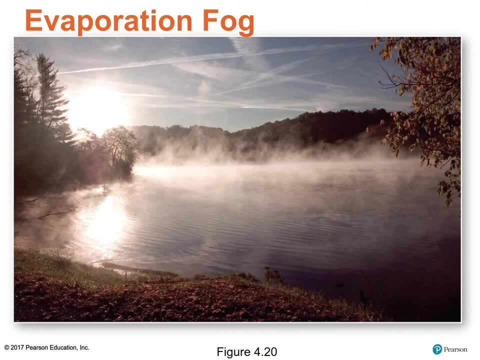 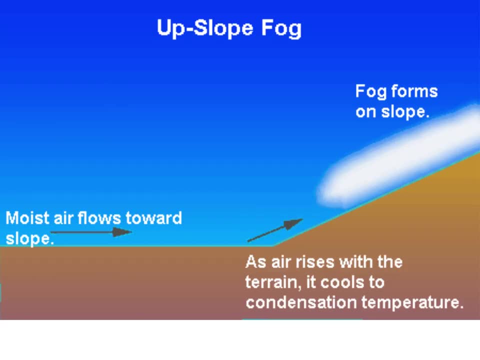 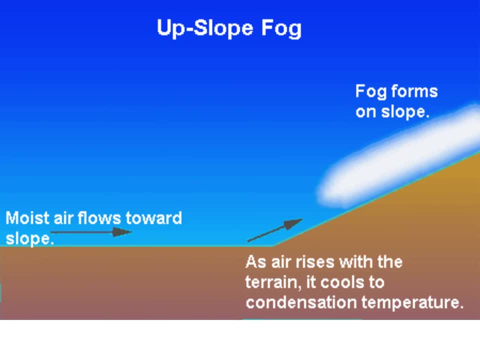 It's orographic lifting. The air is getting lifted because it runs into a physical barrier. it's the same process that creates lenticular clouds when the air gets moved up a mountain. That's called orographic lifting. So you've got warm, moist air. it gets lifted up. it cools instead of making a cloud. it's. 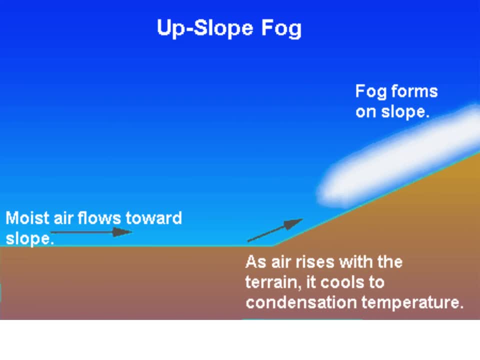 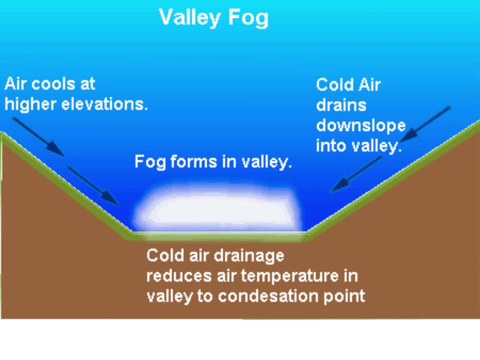 on the ground, so we call it fog. The opposite of upslope fog would be valley fog. With valley fog you have a valley and on the sides of the valley it gets cold. As it gets cold, the air gets more dense and it flows downhill into the valley where 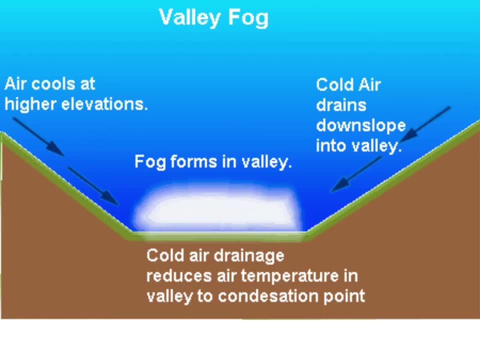 it mixes with the warm air, cools it and makes fog. So it's a density current of the air sinking downhill because it's colder and therefore more dense than the air around it. Puddles in the valley makes fog. Here's the Grand Canyon on a foggy day. 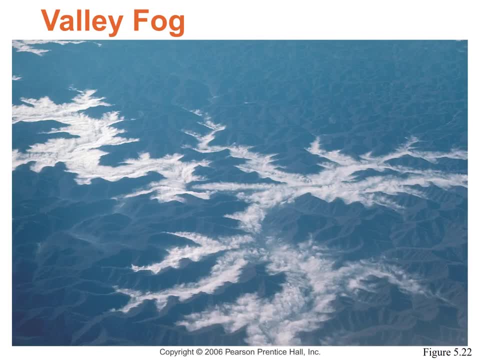 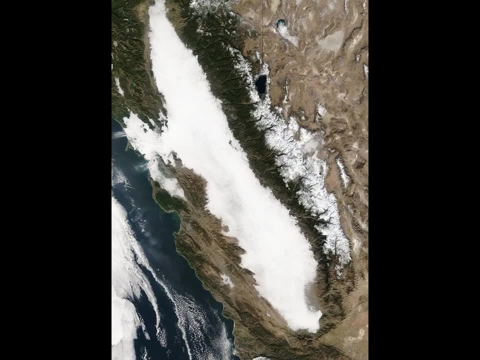 This again is valley fog, where you can really see that the fog is just down in the valleys. We get valley fog and on this day the thickness of the fog it's not too thick because, I'm sorry, scratch that. So here we have more valley fog and it's a very thick fog belt and you can tell. 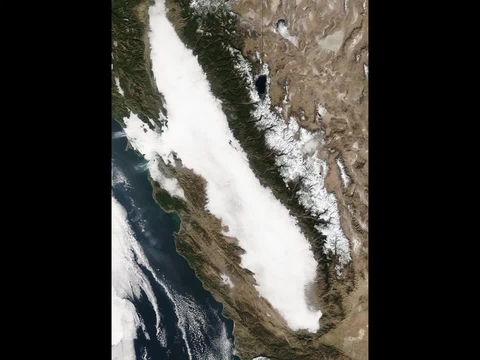 it's thick because you can't see the sun. You can just barely. I don't know, maybe you can see the Sutter Buttes just a little bit. On days when the, when the fog is thinner, when it doesn't go so far off the ground, you can see just the top of the. 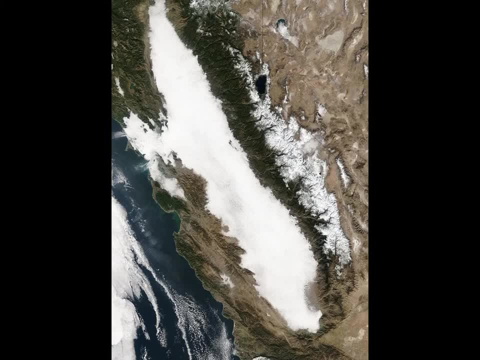 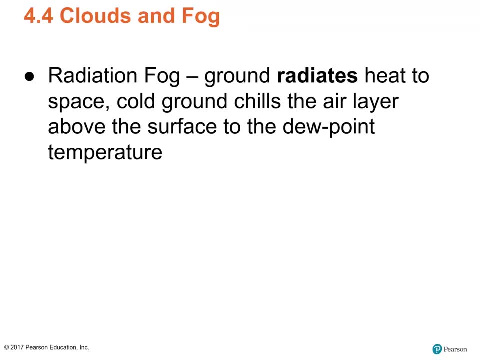 Sutter Buttes sticking out above the fog belt And then you can see snow over the Sierra Nevada. Radiation fog is formed when the ground radiates heat and gets cold. I would call this, personally, cold ground fog, because that's a much better term. That's what it's actually caused by. 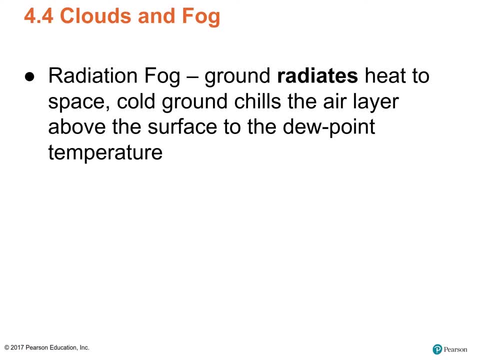 The mechanism is radiation, but people get confused with like atomic stuff. so I'm going to call it radiation fog, but in my head I think of it as cold ground. fog Doesn't occur over water, Remember. because of land, water, heating differences, water cools off slowly. 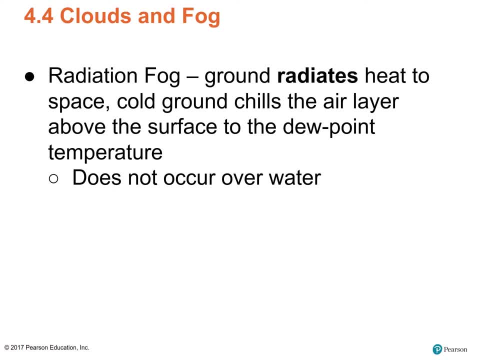 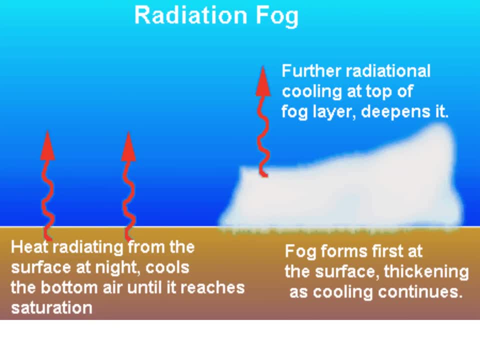 So over water, over water. you're not going to get radiation fog. It's not radioactive, So heat radiates from the ground. You got to have a clear night, Can't be over water, but the ground radiates heat. The ground gets cold. 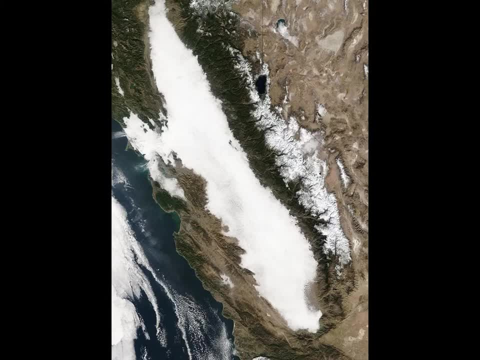 You get fog, Radiation fog. The Central Valley is a wonderful place for fog. We have radiation fog, we have valley fog and also, because of all the agriculture, we also get a little bit of evaporation fog thrown in for good measure. So if you really like fog, the Central Valley is a great place to go. 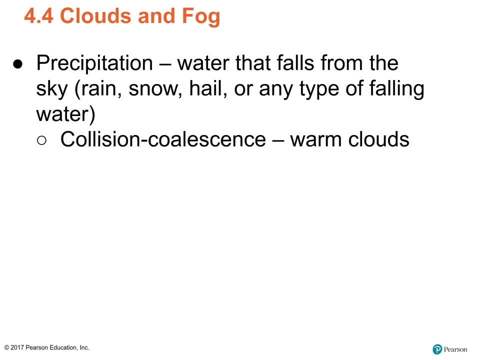 Precipitation: Again, it's water that falls from the sky. There are two mechanisms that make rain. One of them is the collision coalescence mechanism, and that occurs in tropical clouds- Clouds where the temperature is above freezing- and the Bergeron-Findyson process in clouds that are below freezing. 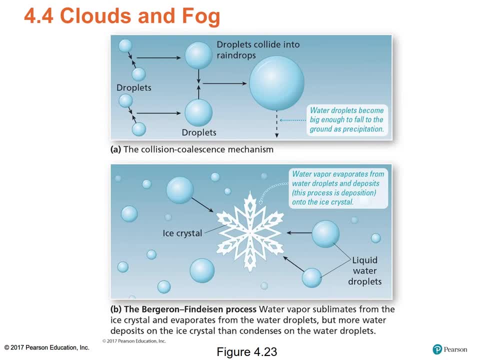 So the collision coalescence mechanism. I think it's really straightforward. You have little droplets of water. They bump into each other to make bigger droplets. Those droplets bump into each other to make bigger droplets. Eventually you get a drop that's big enough to fall from the sky. 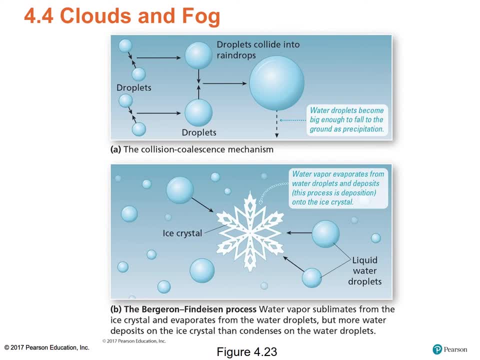 That's the collision coalescence mechanism. That's what makes tropical rain. In colder places, like all the rain we get, it starts as snowflakes. So because the relative humidity is higher over ice than it is over water at the same temperature. 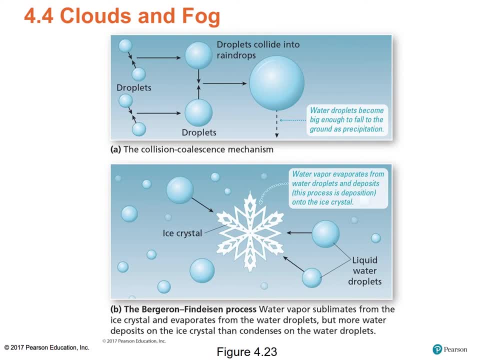 water vapor is going to deposit onto the ice crystal rather than condense out onto either a condensation nuclei or an existing droplet of water. So you've got water- water molecules sublimating off of the ice and depositing back on the ice. You have water. 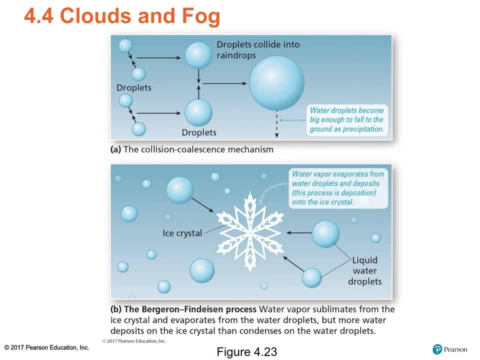 molecules evaporating off of the water and condensing on the water. But the overall trend is that more of the water molecules will sublimate out onto the ice crystal. So the water droplets are going to get smaller and smaller and smaller. The ice crystal gets bigger and bigger and bigger. 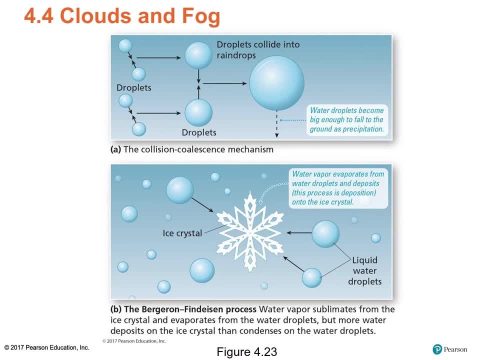 until it gets large enough to fall. In the winter time the air under the cloud is warm enough to, So we just get it as drops of water. We get rain, But all the rain that we get in the wintertime starts off as a snowflake in the cloud. 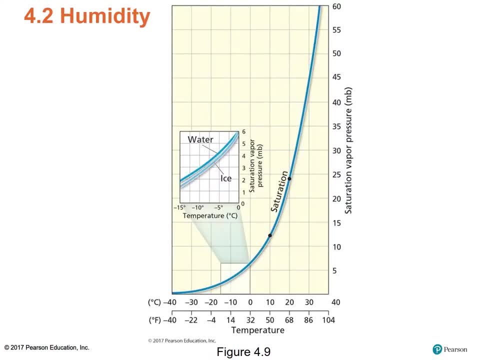 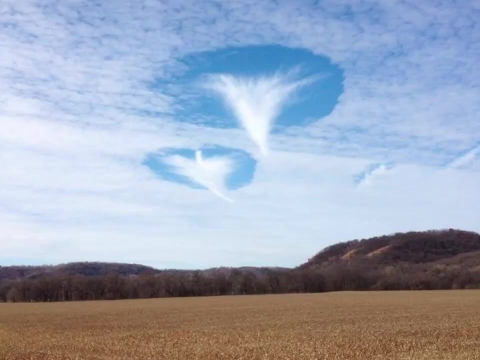 So here's a chart showing the saturation vapor pressure, which is another way of looking at humidity. So here's a chart showing that relative humidity is higher over ice than it is over water. This also creates fall streak or hole punch clouds. So what's happening is you've got an altostratus cloud. 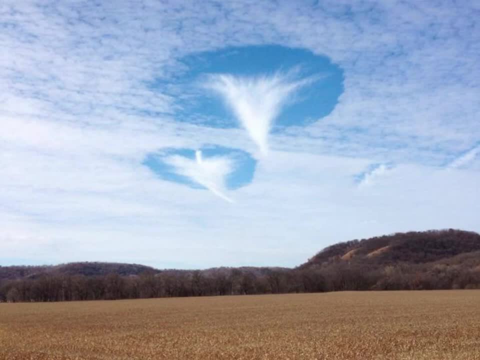 It's right about freezing. So the cloud, the droplets are going to be made of water that's close to freezing And you've got ice crystals. So what's happening is the water vapor is evaporating, It's sublimating out onto the ice crystals and then the ice crystals are falling from the sky. 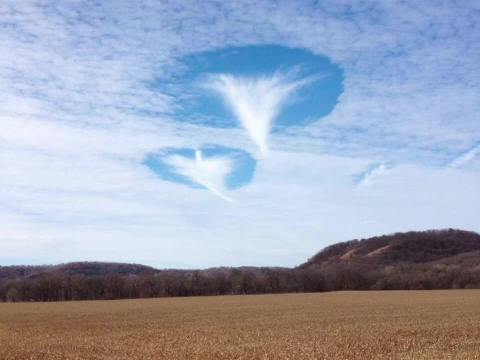 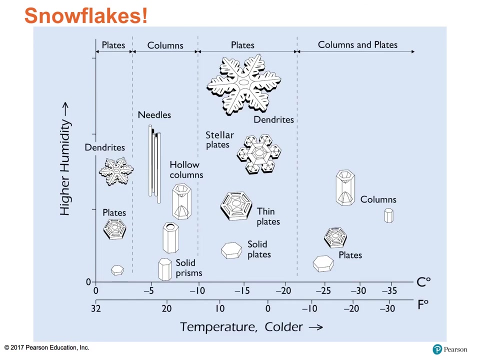 So over time the hole is going to get bigger and bigger and bigger as the water evaporates and then sublimates out onto the ice crystals, And those again are called clays, Hole punch clouds or fall streak clouds. Speaking of ice crystals, the humidity and the temperature determines the shape of ice crystals or snowflakes. 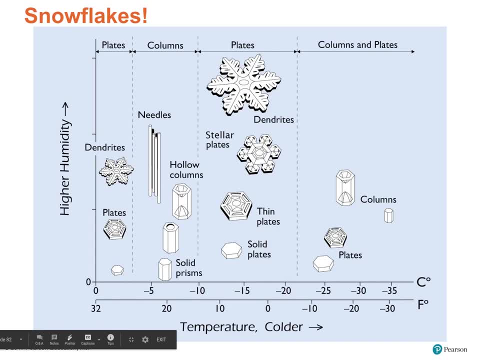 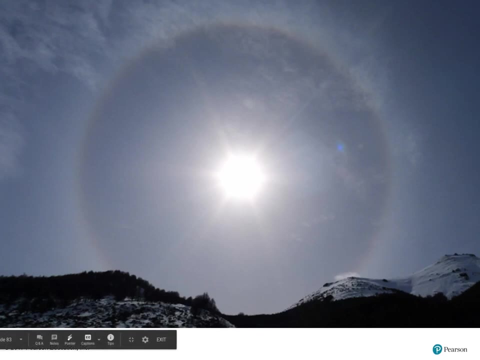 Depending on the temperature and humidity, you can get needles or columns or flakes or plates, And all of those refract light. They bend light. They are why ice crystal clouds have this distinction. They have a distinctive corona or halo around the sun or around the moon. 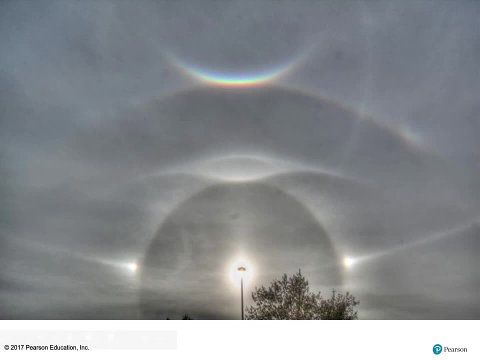 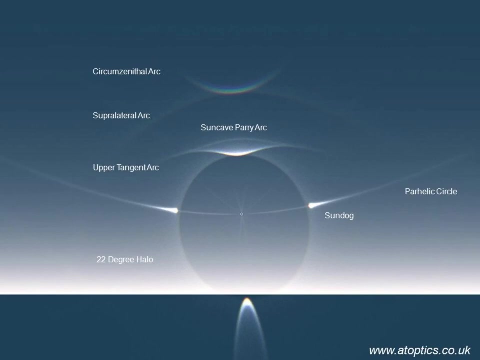 This is just an amazing photo. This is a sun dog. This is a sun dog. The two bright spots on either side of the sun are called sun dogs, And here's a chart showing you the different names for the perihelix circle, the sun cave, peri-arc, the upper tangent arc, the supralateral. 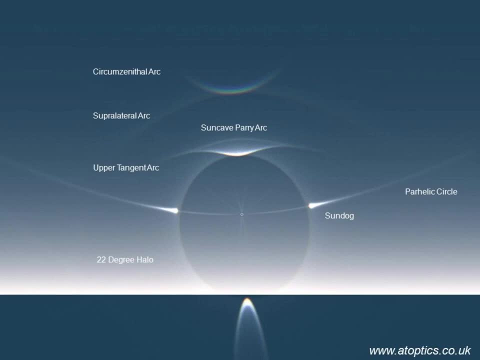 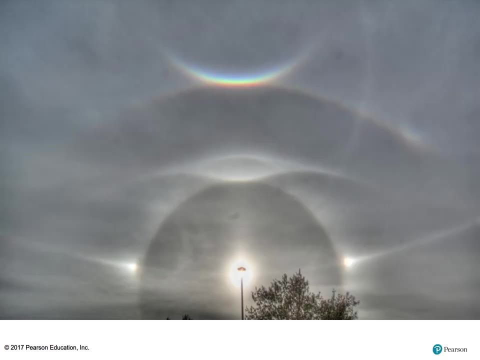 I'm not going to quiz you on any of this stuff, but it's kind of cool that people have figured out names for them all And this diagram is really, really close to this actual picture. Oh, including these little weird things. Man, what an amazing planet. 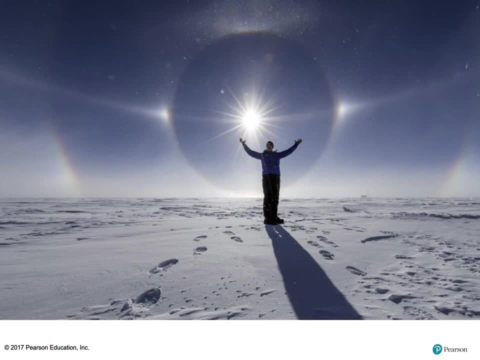 This one. this picture is taken, I believe, in Antarctica, And in it you can see two halos, One halo, two halo 22 degrees away from the sun, 44 degrees away from the sun. Here we have more Virga. 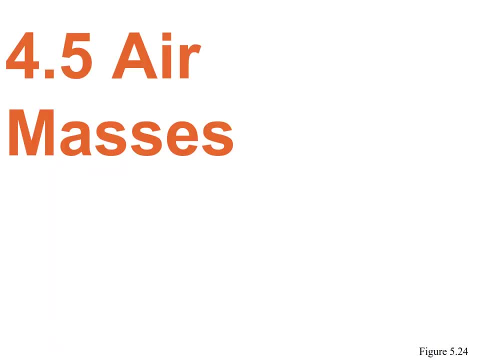 I believe this is in Alaska, And now we're going to talk about air masses. So with air masses, the name tells you everything. There's a system for naming them. The first letter is lowercase. It tells you how humid that air mass is. 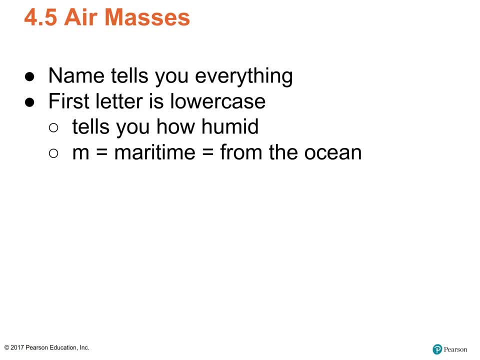 You've got your two options: M for maritime, And those are air masses from the ocean, So they're moist. You can even remember that as M for moist, C for continental. Those air masses are found inland, They are drier. 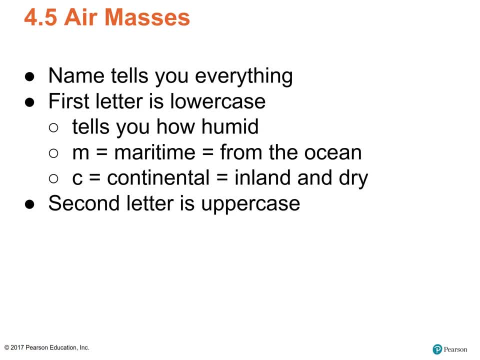 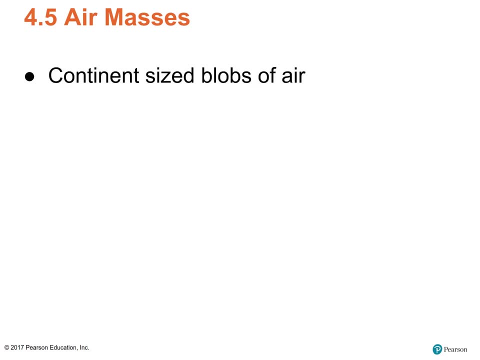 Because the land is not made of water. The second letter is uppercase. The second letter tells you the temperature. We have T Capital. T for tropical, Those are hot, P for polar Cold And A for arctic, Those are super cold. 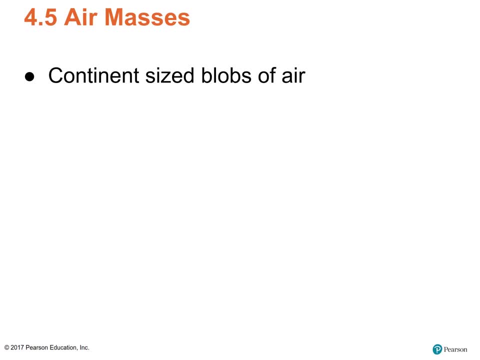 Air masses are continent-sized blobs of air. I'll show you a diagram in a minute. You can see just what I'm talking about. They extend up through half the thickness of the troposphere, So up to about 6 kilometers or so. 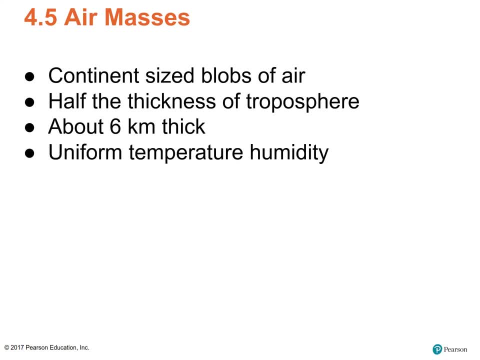 They have uniform temperature and humidity. So throughout the air mass, the temperature and the relative humidity and the specific humidity, it's all going to be about the same. When two different air masses meet, they don't mix, They form a front at the boundary layer between them. 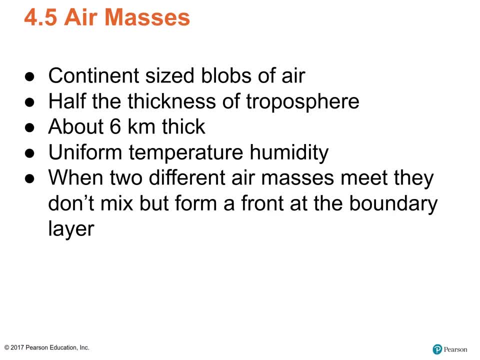 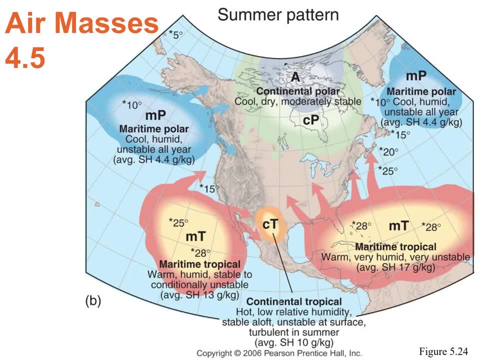 Cold fronts, warm fronts- we'll talk about that later when we talk about weather in this chapter. And here's a diagram of summer air masses: So little M, big P, maritime polar, So we know that it would be cool and moist. 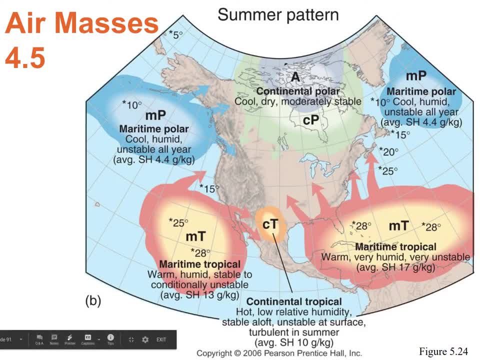 Maritime, tropical Maritime- would be moist, So that would be really warm, really moist In fact. specific humidity of 13 grams. Over here in the Gulf of Mexico, the Caribbean, the water temperature is higher, So there's more evaporation. 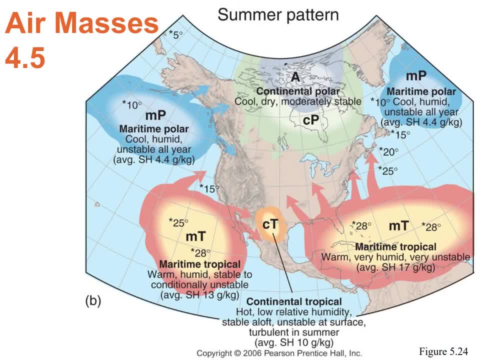 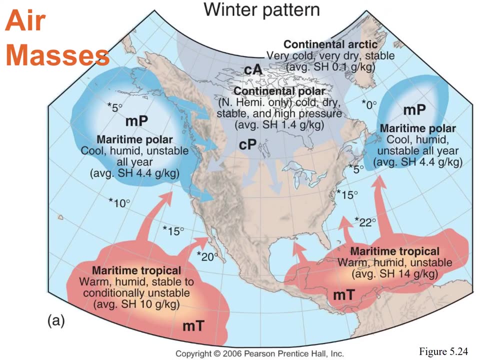 So the air masses there are going to be more moist, at 17 grams Continental polar, 4 grams Maritime polar, 4.4 grams Cooler, Dryer. In wintertime we can develop continental arctic air which is incredibly dry. 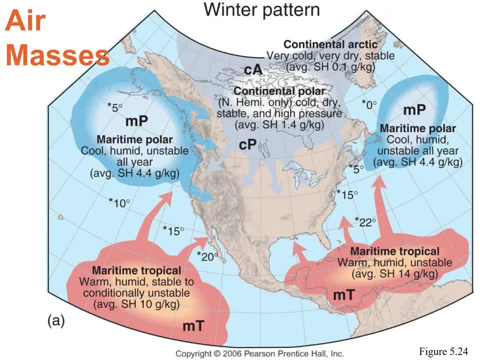 0.1 grams of water vapor per kilogram of air. In California we deal with maritime polar and maritime tropical. If we lived in the Midwest or in the Northeast, we would be dealing with continental polar or even continental arctic air. 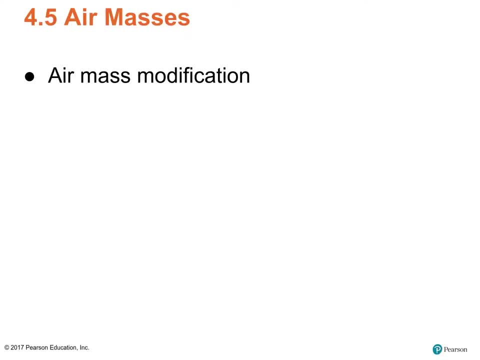 which would be much, much, much colder. As air masses move along, they gradually change. So when they start out, for example, that air mass over the ocean, it's going to be the temperature, it's going to be the humidity. 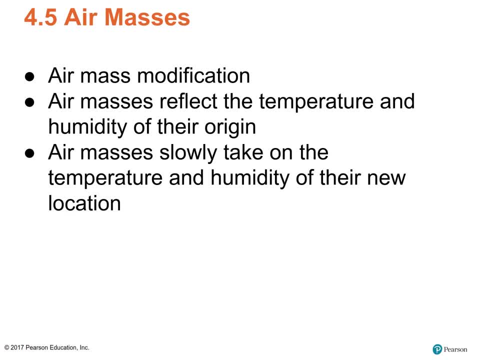 it's going to reflect the characteristics where it started As it moves inland. it's going to get lifted up, it's going to cool, you'll lose water vapor, so it'll get drier and it'll gradually take on the characteristics in terms of temperature and humidity. 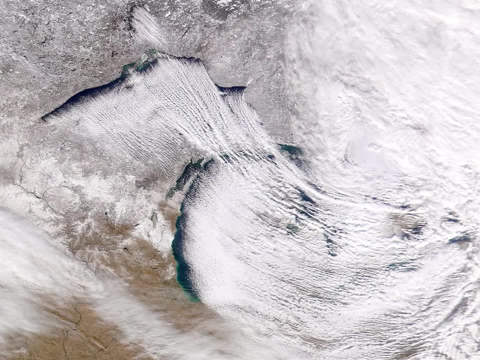 of the new location. So over the Great Lakes in the winter time you have these very cold, very dry air masses moving over, and as they move over the Great Lakes evaporation is occurring, So the air masses pick up water vapor. 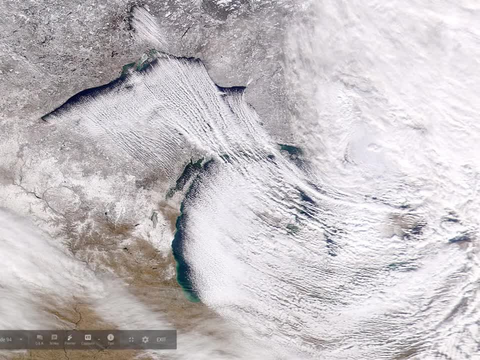 and then you get condensation and clouds downwind from the lake. So upwind, like right here is Chicago, nothing going on there. downwind looks like they're getting lots and lots and lots of snow. So if we look, for example, at Chicago,